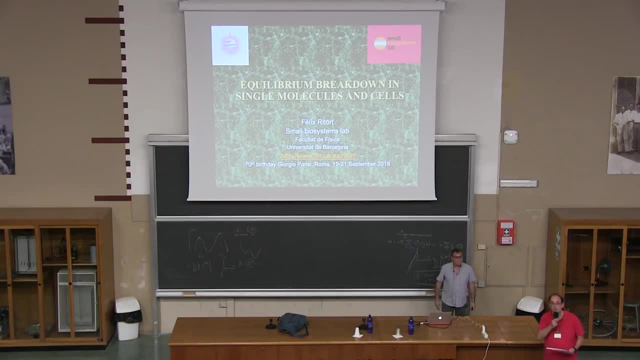 Good afternoon, everybody. We will start the next session. It is a pleasure for me to be here celebrating the anniversary of Giorgio. I have been working with him the last 25 years and it has been also a pleasure. Thank you, Giorgio. The first speaker is Félix Ritor. 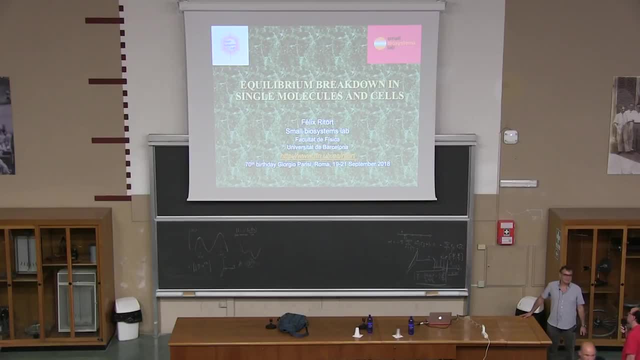 from Barcelona University. We will speak about equilibrium rectums in single molecules and cell. Please. Thank you very much, Juan Jesús. Good afternoon everybody. It's a real pleasure to be here to celebrate the 17th birthday of a great person such as. 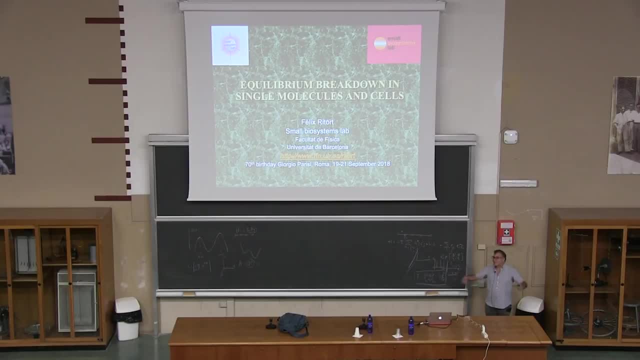 Giorgio Parisi, and everyone has to start telling something about his experience with him. So I am a privileged one because my story starts in 1989. but actually when I started working with him was in 1990, when I came to Tor Vergata. He was at that. 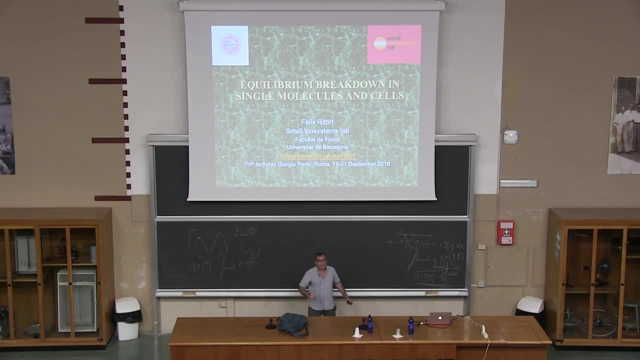 time at Tor Vergata and I was privileged because I was sharing the office with him. Okay, so everyone, when you are very young- you are 23,- you are put in an office with the other students, but he told me so he put me in his office and I had a great opportunity to have conversations with him and also 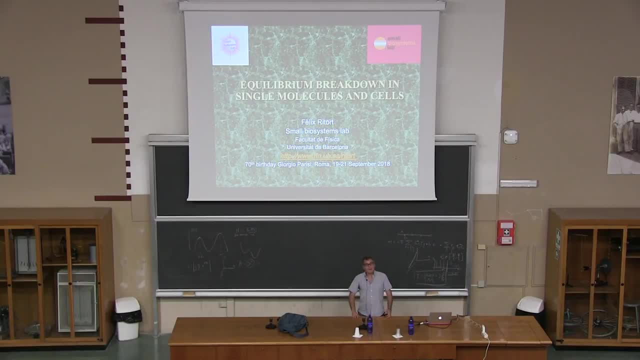 I think I helped him a lot because many people wanted to speak to him. so what they did they do at that time we had Bax, which was a computer system, so they sent me a mail, a message. Félix is Giorgio there, Giorgio in the stanza, is in the room. I said, yeah, you may come now and then. 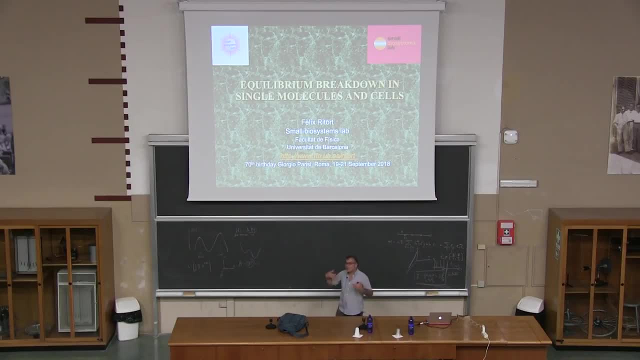 they came and they looked for him. So all the time people was contacting me to know whether he was in the room or not. okay, and, as you know, this is good because Italy is a country of favors. So if you so, if you give a favor to someone, then they can give it back to you. okay, but yeah, mine for sure, yeah. 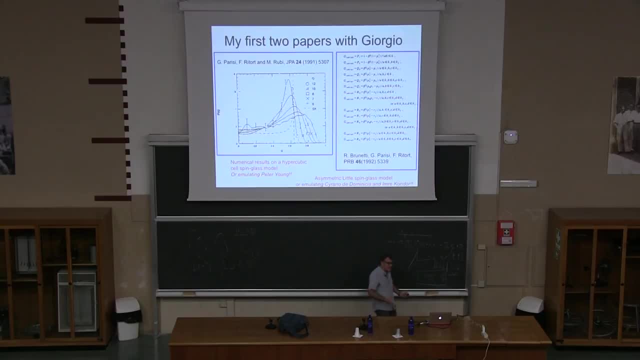 so, going to the more scientific part, these are my first two papers with Giorgio, which I put here because I looked at them this morning I said I like this work. this was beautiful work. of course, these were my first papers. it was a lot of work, okay, so 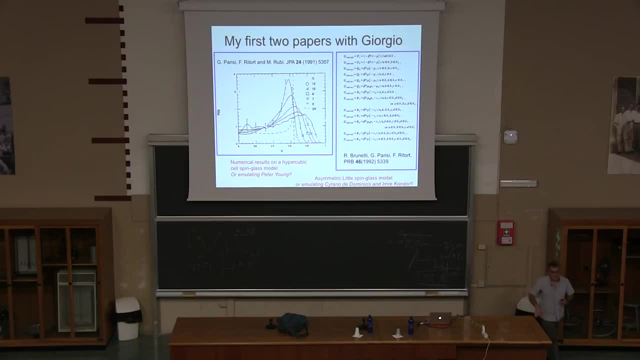 my first paper was doing something that we have heard about Victor Martin Major yesterday, and also Juan Jesus has been working a lot, which is numerical simulations of spin glasses, and my lead, my, my idol that time was Peter Young. Peter Young was so good making simulations in field in finite dimensions, and we studied this hypercube which is a. one dimension is a. 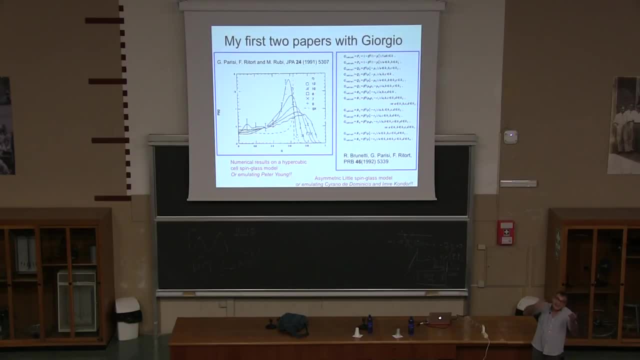 many-dimensional single cell unit and, of course, as an hypercube, as a single cell has a number of sides of spins, which is two to the power, d, and when you increase d, you increase the number of spins and you increase the dimension at the same time. okay, it's a mean field model and but you cannot solve it exactly, even if it looks at a very 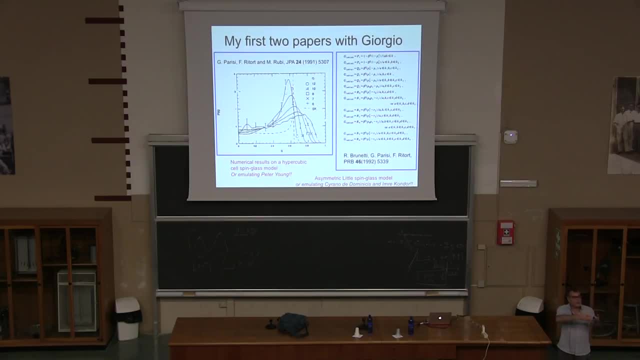 simple model. it's not like the sharing donker patrick model which you can solve analytically in the hypercube. you don't have links everywhere and you cannot solve it exactly, but it's fully connected somehow and we find this p of q for the other parameter. i had another experience at the same time, which was the second. 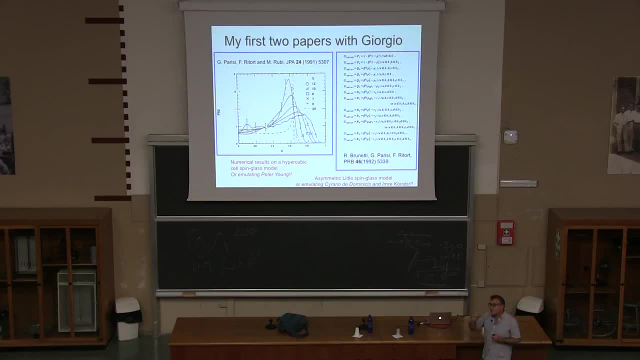 paper. i work on a model which is called a little spin glass model, which is like the sharington kilpatrick model, but putting interactions between two, let's say two bipartite lattices. so it's the same hamiltonian as a sq model, j, sigma, sigma, but now you have sigma tau and you. 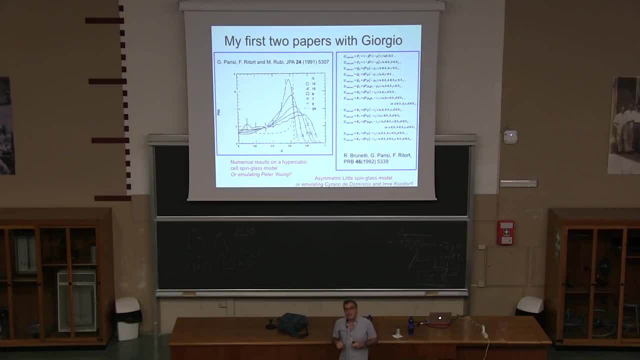 make connections. j sigma tau. okay now, it was a hard work because i had. the goal was to demonstrate that this is exactly the same as the sharington kilpatrick model. but the demonstration is not clear at all and what i was able to demonstrate is that, at first order of relic, asymmetry breaking. 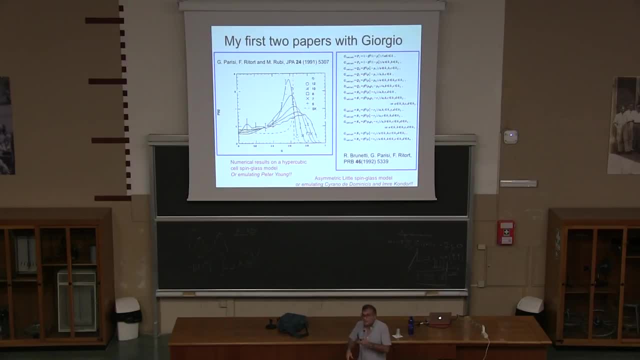 the little model and the sq model give the same free energy. but for doing that i had to diagonalize a very complicated stability matrix, okay, and. but at the end i succeeded. and i was also, of course, i admired the talent of Cyranoid Dominicis and Imre Condor, who did this, of course, 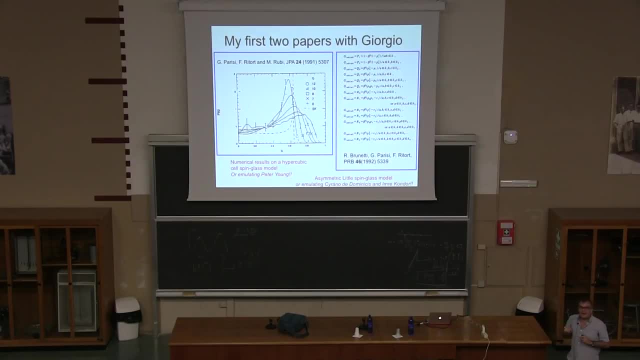 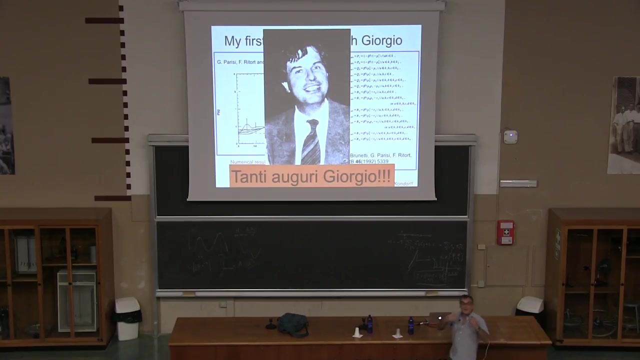 in the whole spectrum. i did just at first of the replica symmetry breaking. but that was very nice, this work in simulations and this work on theory. so what i want to say is: thank you, georgio, thank you very much for everything you have given me, not only to me, but all of us. okay, but now life. 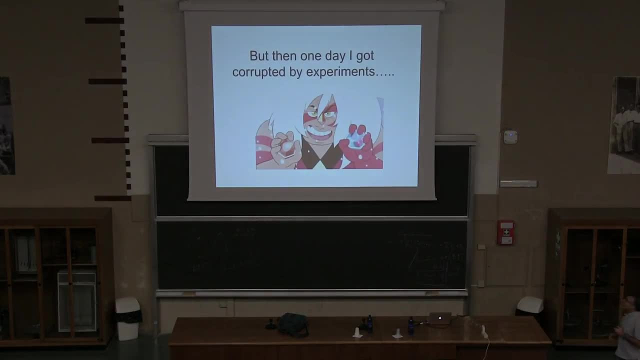 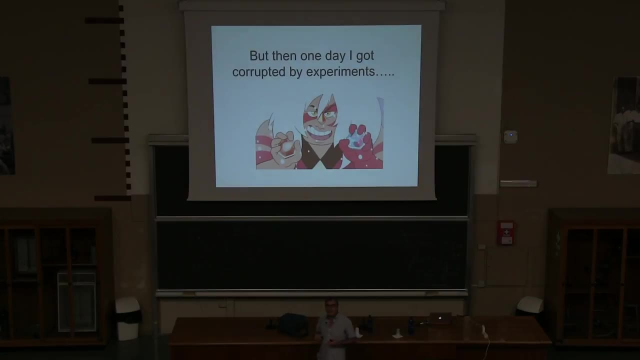 is never perfect. and a few years later i got corrupted by experiments- okay. and then i decided to learn about doing experiments- okay. so i had already an experience of 10 years in theory, first in spin glasses, and in glasses said no. now i want to see the truth. 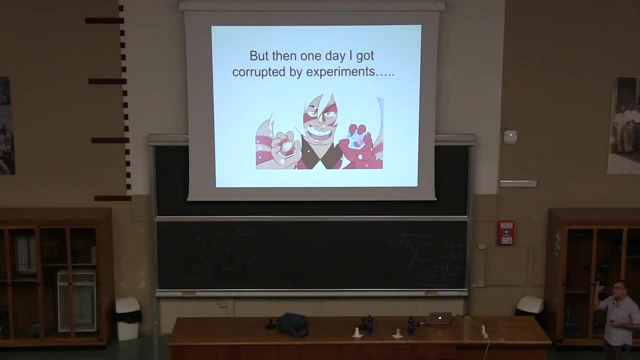 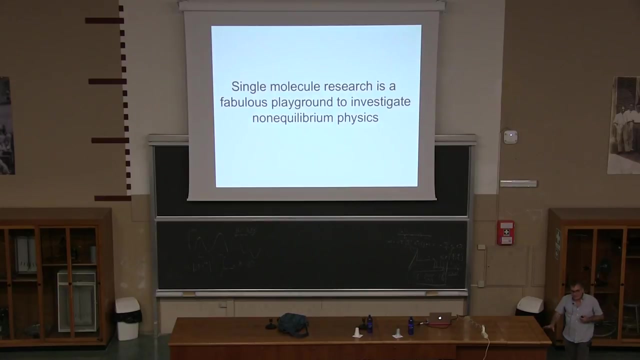 i want to see a nature. i want to see what nature shows me in an experiment. of course, georgio is extremely smart, but they wanted to go further, and nature is an absolute master. okay, so what i'm going to show you today- and i go to the key to the center of my topic- is about studying. 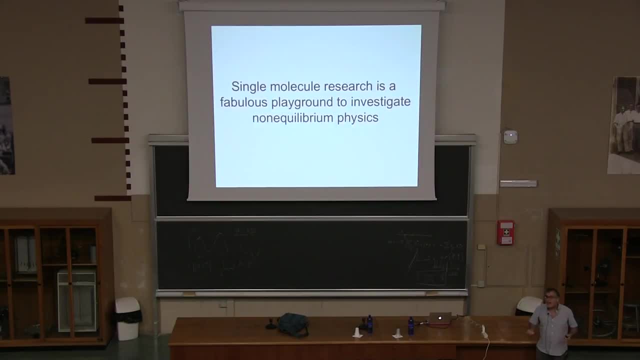 about the studying, if you want, disordered systems, statistical mechanics of complex systems, non-equilibrium physics, using the playground of small systems, okay, and what i want to demonstrate or convey to you is that small systems- when i think of small systems, i mean molecules- can be molecules of 10, 20, 30, 40, 50 monomers, i don't know, but small systems at the molecular. 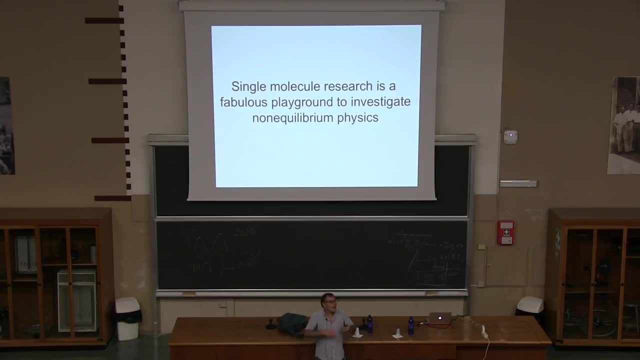 level also behave, share all these properties that we are studying in the molecular system since the sharing, sharing donkey patrick model and beyond. so they are a fabulous playground to investigate the problem about disorder and fluctuations. okay, so one of the problems i have been working over the past years: 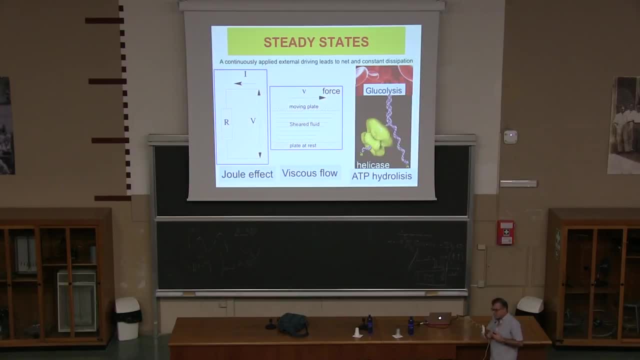 and actually was introduced by. in the previous lecture by stefano rufo, he talked about these non-equilibrium steady states, so systems that to keep them on you need to supply continuously power. okay, and these systems are very interesting because they are time stationary, so the properties are not changing time, but still they are out of equilibrium because you pump. 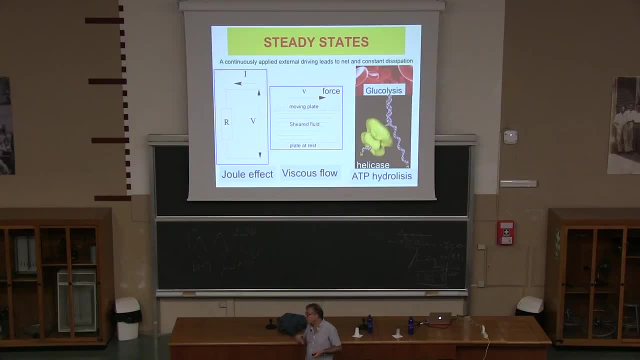 some energy which in average is taken out to the bath in the form of heat. so they are continuously producing entropy. they are out of equilibrium. of course they cannot be described by bosman gibbs distribution. so there are different examples. one is a current through resistance. there's a 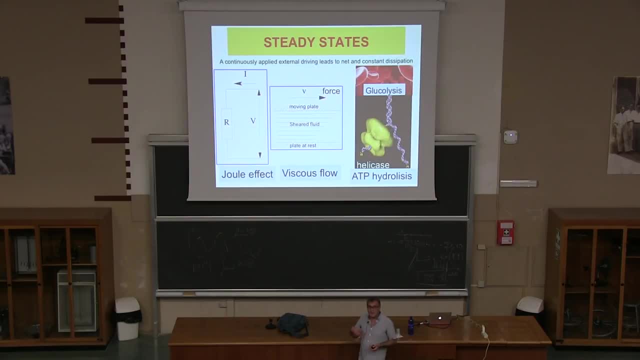 jaw effect. you need the source of potential and then you have this steady state of the electron flowing through the resistance. you can also produce a non-equilibrium steady state by taking a fluid which is an equilibrium and then shearing one plate with respect to the other. the constant speed you produce, you exert an external power which is 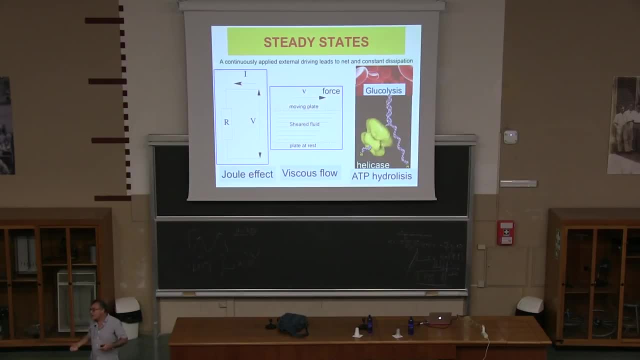 the average force due to friction times, the velocity, and this is, in average, dissipated in the form of heat to the environment. okay, so these are isothermal systems and these- the other ones are the ones that interest me possibly most- are related more to biological systems, which are for 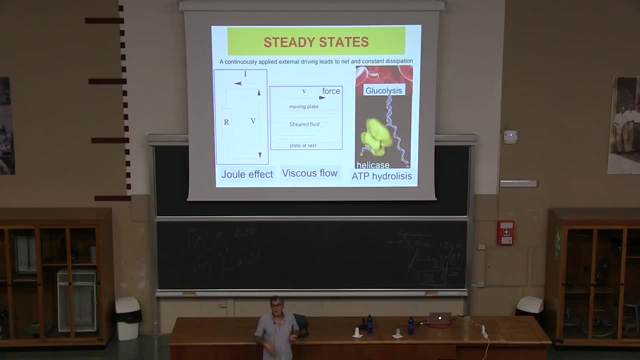 example, chemical reactions that drive molecular motors across a substrate. and here is an example of a molecule called elegase. it's a protein that unzips dna separated to strands by using ATP hydrolysis. it's a steady state. okay, you open the dna double helix continuously with a. 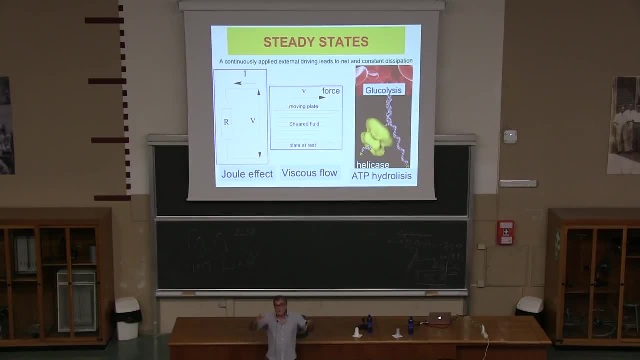 constant speed as a function of time. another example is a living cell, and here i show you an example of living cell, which is a red blood cell which is not living, because red blood cells are considered to be alive- okay, they are. just, if you want, chemical bugs that experience some. 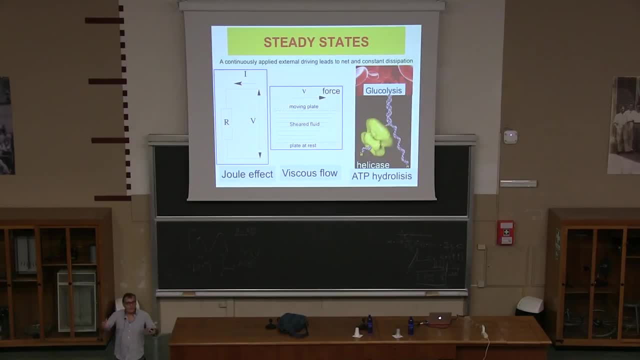 metabolic processes and they evolve, but they don't reproduce, they don't, they don't duplicate and so on. so they are not considered living. but these are more close to active systems, possibly a living system, but still these use sugar from the water in the solution, the glucose, and there are process 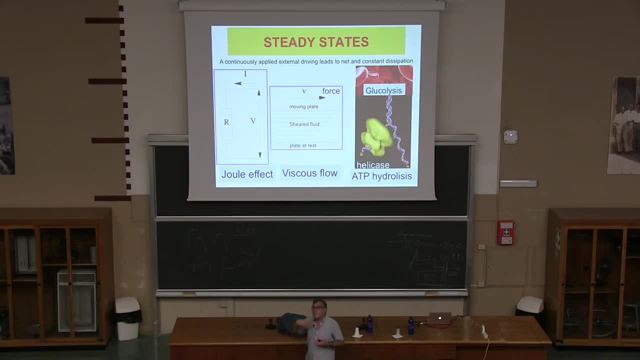 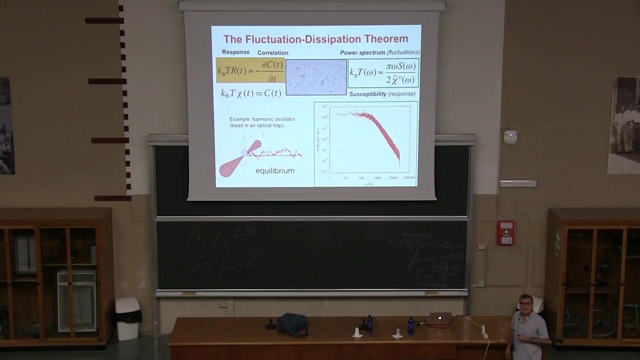 metabolic process inside the red blood cell that make them maintain some sort of metabolic state. these are very interesting also non-equilibrium systems, steady state systems, for the reasons that i will indicate after. so one of the results that um have been much studied in our field of disordered systems and spin glasses, and 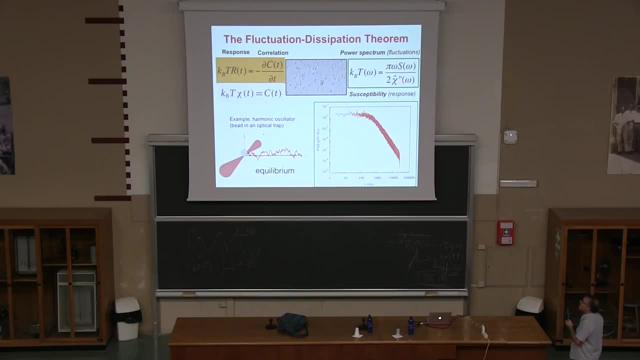 and so on, is the fluctuation dissipation theorem, which i will remind just for those of you who maybe don't remember the details. it tells you that, basically, a system in equilibrium, fluctuations decay in a way indistinguishable. spontaneous fluctuations decay in a way which cannot be distinguished of. 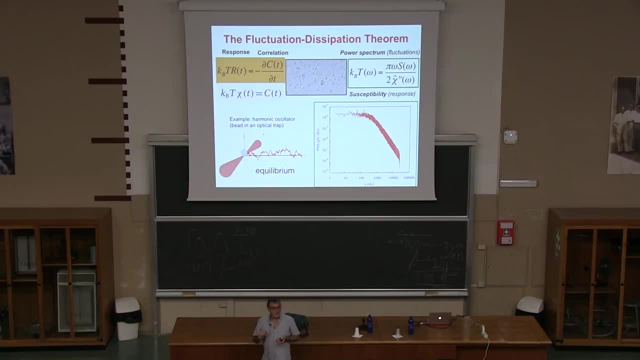 an induced relaxation, for example by perturbing the system. so if i take a particle and move it, i push on it. that motion induced by the force that is pushing is indistinguishable from a spontaneous diffusive motion without force. basically, it says that and it connects the correlation function to the response function. this is a so-called differential. 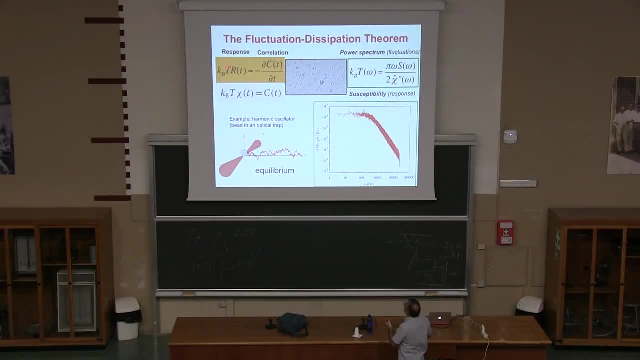 form. and if you integrate the response and the correlation, then you get, of course, for the response, susceptibility and it tells you that the integrated response equals the correlation. i have written in this way. okay, there are different ways to write. it depends how you define the correlation function at zero and so on, but this is basically the thing you have, also the. 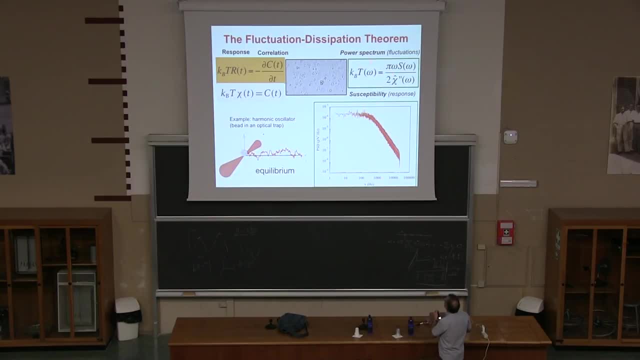 same relation in frequency space and you have to relate the corresponding quantity in frequency space to the correlation function, which is a power spectrum s of omega, to the equivalent quantity in four year space of the response transform, which is the out of phase susceptibility. so if you drive your system with a finite frequency, the system has a lack behind the driving force is lack. 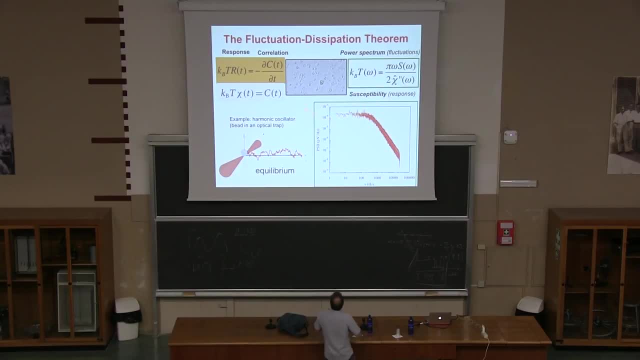 which is this. the facing defines the autophase, susceptibility, and you can measure experimentally these quantities, for example the power spectrum. nowadays there are a lot of experiments in beats, in optical traps, and here, even in rome, you have experiments. for example, there's Roberto Leonardo. THAT IS THE TROOPER 바� Tages Beautiful thing. in the past I found all this is themed startling. First part of the movement of constantly shifting current flow, the activity pienouing to centeref, condensation, base air and phase to distribution pressure darит a permanent flow and they can have automatic victory, but unfortunately osaic you'll need space knows also things andığın the way the functions influence the sides, and Engineer of Space, i usually see things like the Class e power spectrum. so 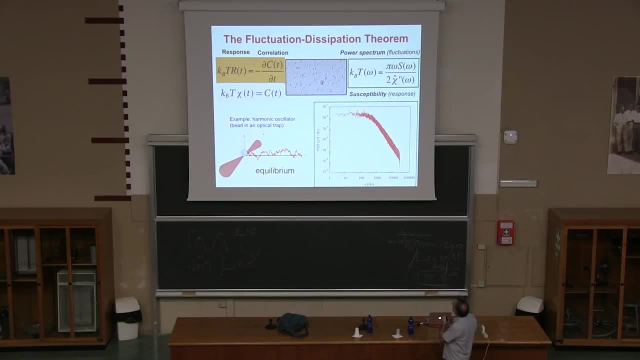 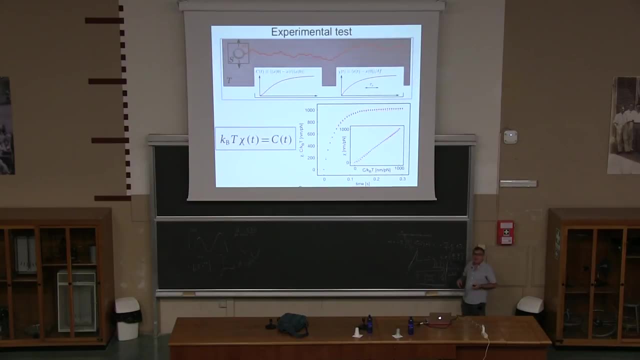 things okay, and he measures this power spectrum and this is a typical Lorentzian. and now you can ask: okay, can I verify my fluctuation dissipation, the fluctuation dissipation theorem, by using this very simple model of a bit in an optical trap. so this bit, 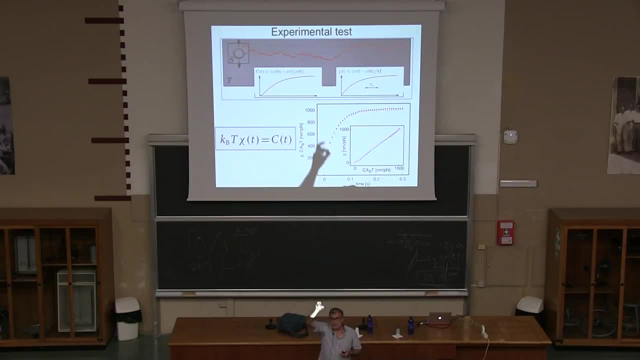 is a harmonic potential. it fluctuates. of course, it's confined to this harmonic well, and I can do the experiment. sure, I can do the experiment. I can take my bit, which is exerting this trajectory, and then I can just keep track of the position along one axis. 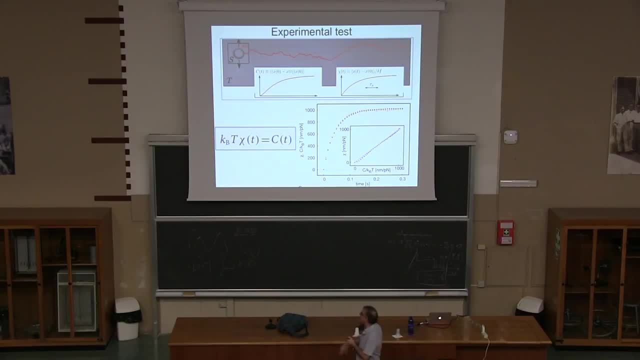 so a bit in an optical trap is three dimensional. I just track one coordinate and then I measure the correlation function, which I define this way. this is just convenient. usually you see x, t, x, 0. I define this way because I want to match the correlation function to the susceptibility. 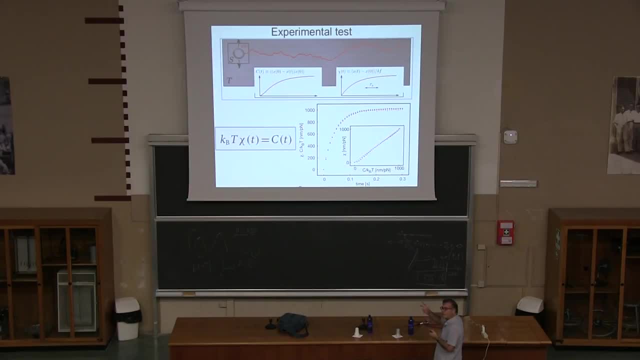 so at 0 time I want the correlation function to be 0. it's just a matter of introducing this x- 0 square here. so it's basically the same correlation function. you are seeing all the time. so you measure the correlation function. it goes from 0 to a maximum value. 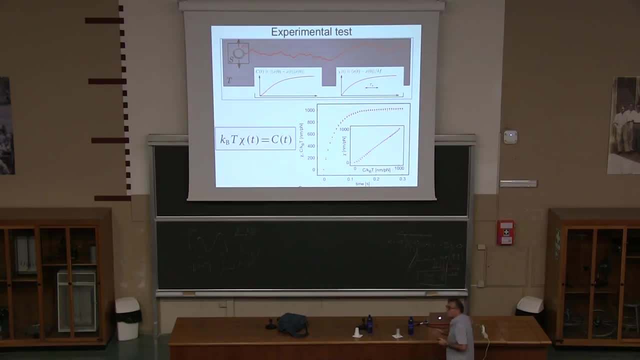 and you can measure also the susceptibility. so the susceptibility is an integrated response function. so for the response you apply an impulse, for the susceptibility you apply a step and then you see after the step how the position of the bit moves. so for example, I take my optical trap. 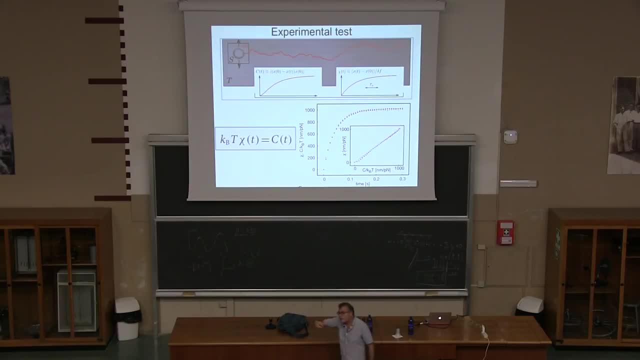 I move by 100 nanometers the optical trap and then the bit follows the center of the optical trap, drag through water, and that trajectory gives me the susceptibility k of t and I put them. if the fluctuation dissipation theorem works, I should get both of them equal. 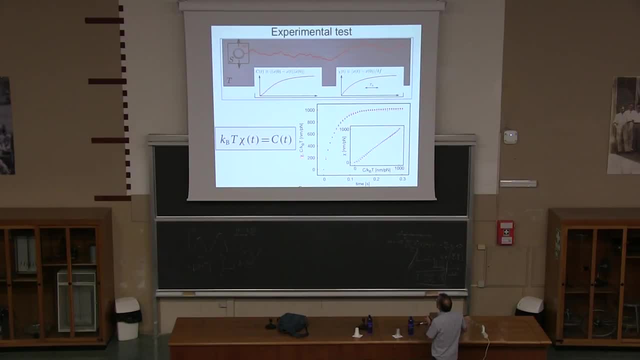 and this is what you see here. these are experimental data on the susceptibility of one of these bits, which is about 3 microns in water, and the correlation function divided by k of t. this is a pure exponential function because of the simplicity of the model, because it's a harmonic trap, it's a linear problem. 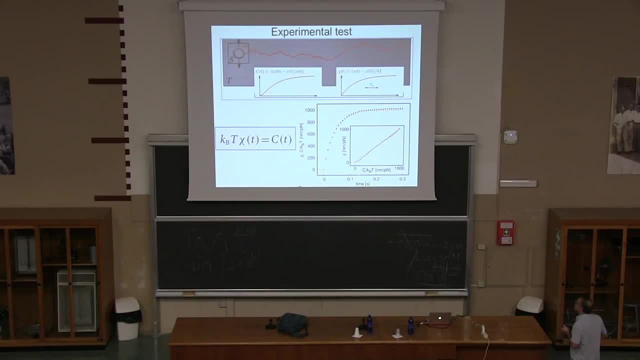 but would happen in any other physical system: the identity between two quantities. so what we do, then, is do something that are called fd plots: fluctuation, dissipation plots. that was a nice idea, actually introduced, from what I know, in the field by Leticia and Jorge. 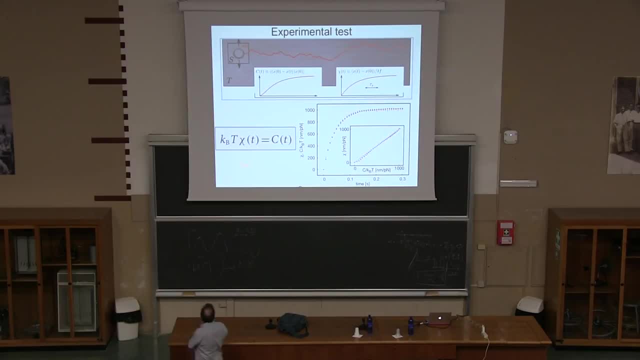 they introduced fd plots and you plot the susceptibility as a function of the correlation and you get a straight line with a slope equal to 1 if the correlation is normalized as a function of k of t, and these are piconewtons per nanometer, because the correlation is nanometers squared. 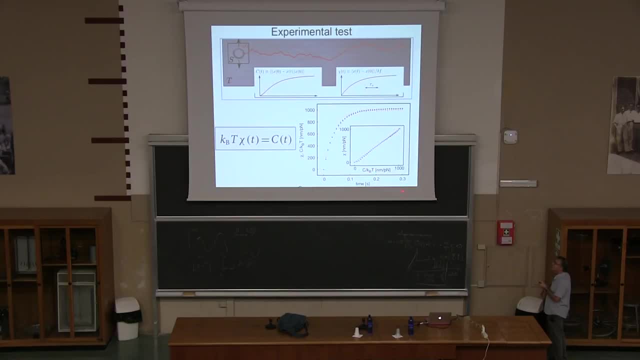 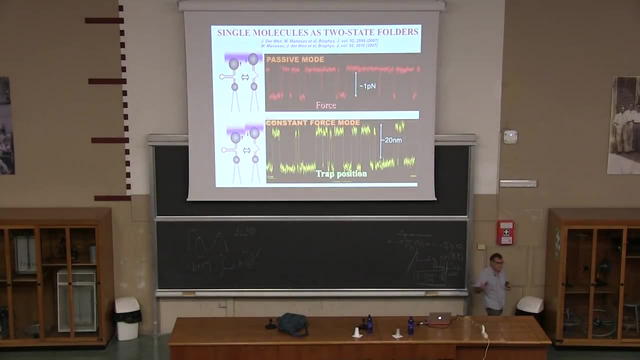 k of t is piconewtons per nanometer. these are the units. So this is the. these are real experimental data. this is for a bit in an optical trap, but I insist, this is independent of the model system. it can be as complicated as you want. 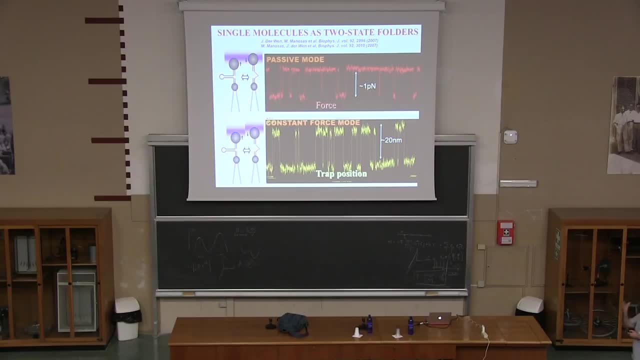 and I can choose, for example, what they call a two state folder, a two state system. so molecule, for example, that can hop between two states. so these are experiments we do in my lab. with an optical trap we have a molecule that can be spontaneously unfold. you tension the molecule. 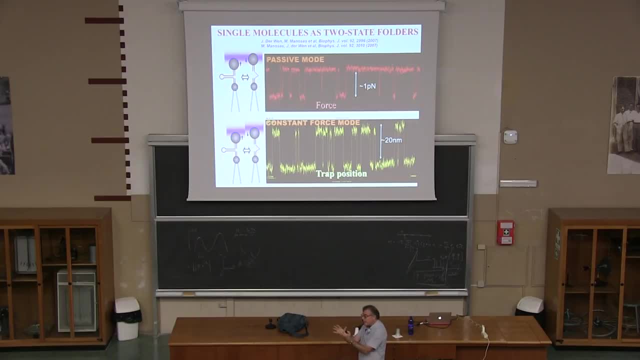 the molecule is always folded. but then what you do is you pull on it up to 15 piconewtons. the hydrogen bonds of the herping cannot withstand against the structure spontaneous starts to hop. it's an experimental realization of dichotomic noise and you have these sort of signals. 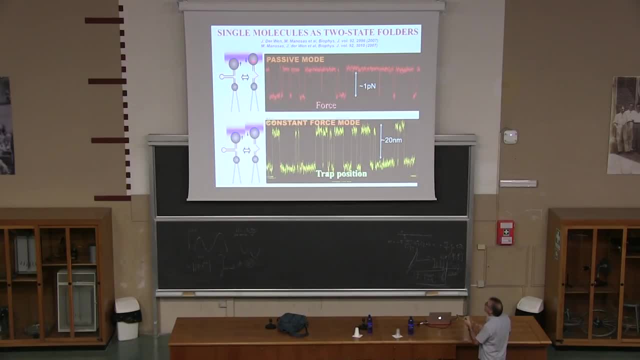 that you can do in the passive mode if you keep the position of the trap constant but the force fluctuates, as you see here. or you can do in the constant force mode if you actively move the optical trap to keep the force constant. but then of course in this sort of feedback 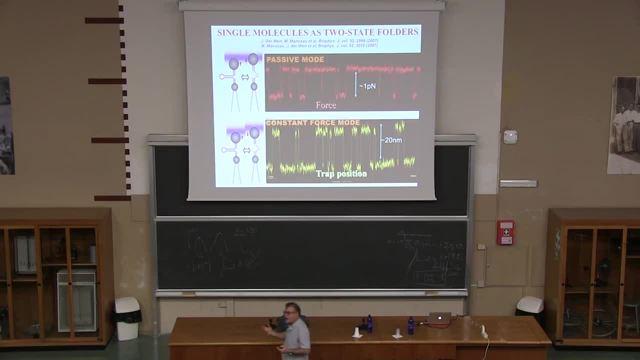 the trap position fluctuates. these are two ensembles of the same problem. if you can experiment with a relaxation analyzing model, you can control the magnetic field or you can control the magnetization. controlling the magnetization is very, very complicated. experimentally no one can do it. 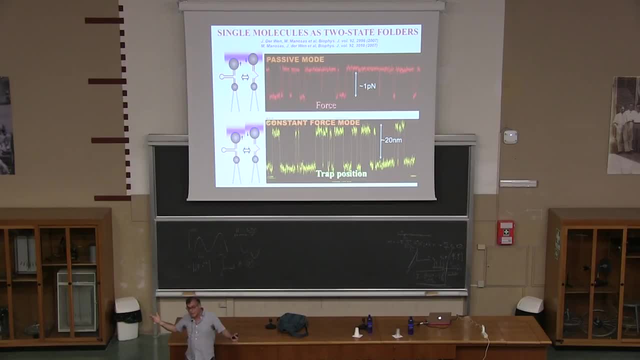 this is the reason why everyone talks about changing the magnetic field. but in principle, why not? you could control the magnetization and see how the magnetic field evolves. this, which is very difficult in experiments for magnetic systems, for single molecules, for my systems is possible, so I have another experimental window. 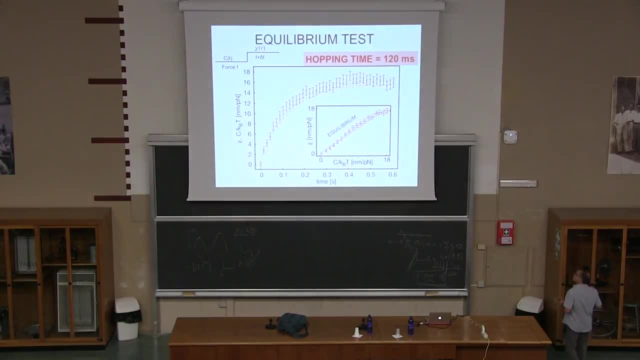 to access what I call ensemble in equivalence, and then you can measure again. in this two-state system you can measure the correlation and the susceptibility, doing in the same way as before: I measure the correlation function, just the correlation function of this dichotomic signal, or I can measure the susceptibility. 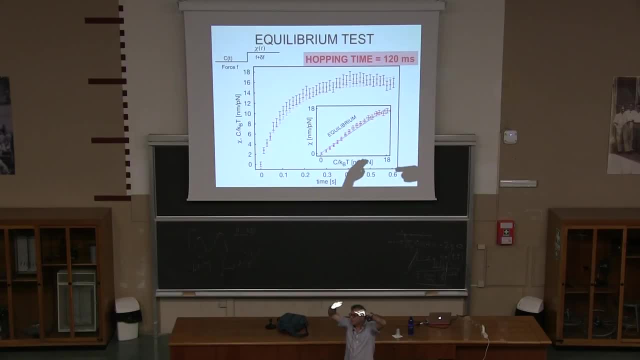 by switching the optical trap, shifting the equilibrium between the two states and seeing how the trajectory that is hopping from one condition changes to the other condition where the probabilities of the two states are being shifted, because the free energy shifts a little bit when you move the position of the optical trap. 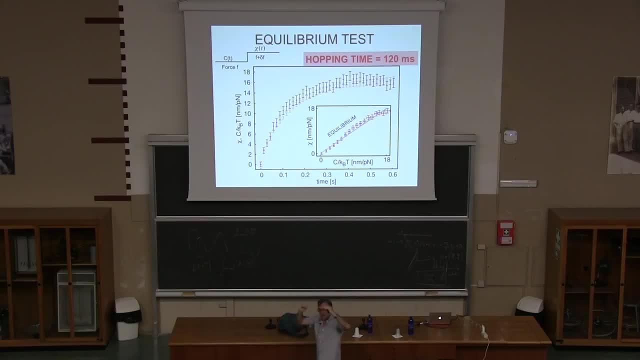 it's like a two-well potential. you can shift it by moving the relative deep, the relative height of the two states. and again you see that this is more difficult to measure, for obvious reasons, because you have to keep track very well of the drift in the experiment. 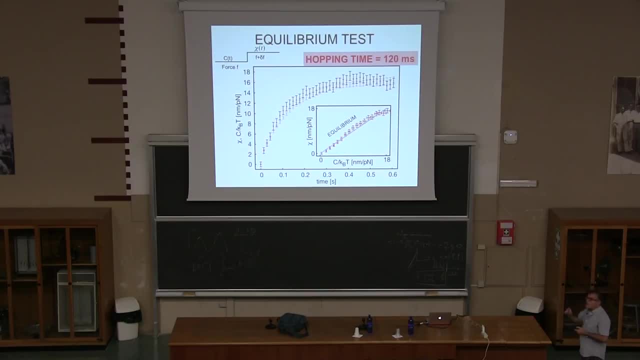 these are molecules that have 20 nanometers of length, that open and close and you are in a regime of non-drift, instrumental drift, that from the beat you can move from microns, basically hundreds of nanometers, so you are much less affected by drift. 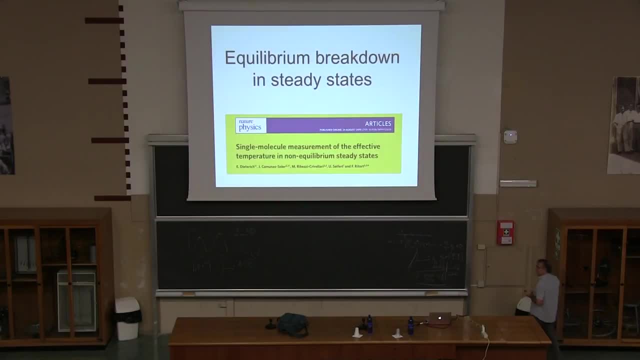 in the other case. that's another case where the fluctuation- and I want to tell you what happens if you put your system out of equilibrium- and of course you know there are several types of non-equilibrium states. the aging state is one of the most studied. 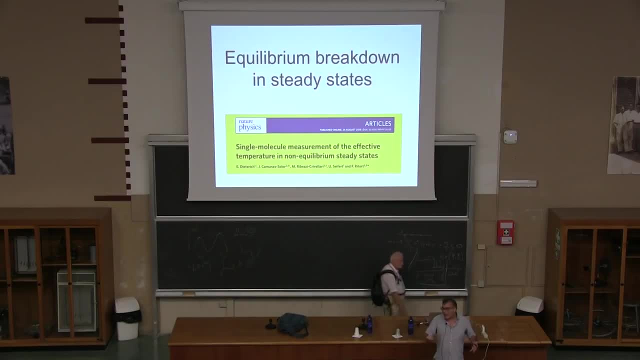 possibly by people here, because it's a natural relaxing state of a spin glass, of a disorder system. but there are non-equilibrium steady states, which means what I showed you before: in the case of the resistance, in the case of the plates, in the case of the chemical reaction. 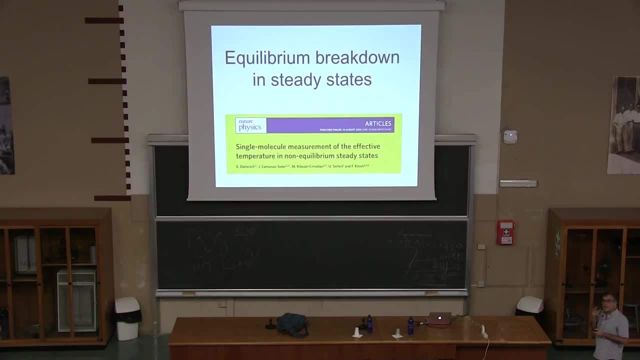 and so on. so the question here we ask is: can we experimentally test the validity of the fluctuation dissipation theorem? and the answer is yes, and you know someone will say: this is trivial. we know that the fluctuation dissipation theorem doesn't work, why do you want to do this experiment? 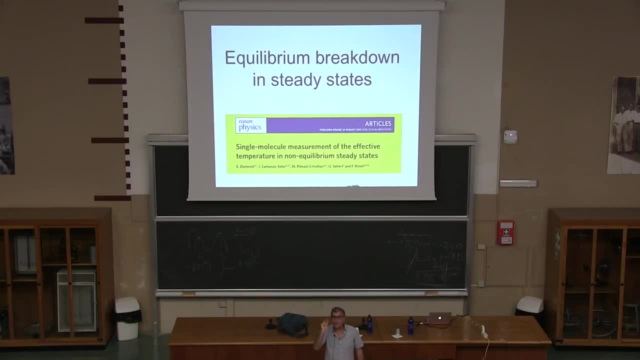 because it's an experiment on a molecule. so I want to use my molecule- one molecule system- to do experiments of what is supposed to hold for big systems in the thermodynamic limit. I have a very small system and to me it was not clear that we had. 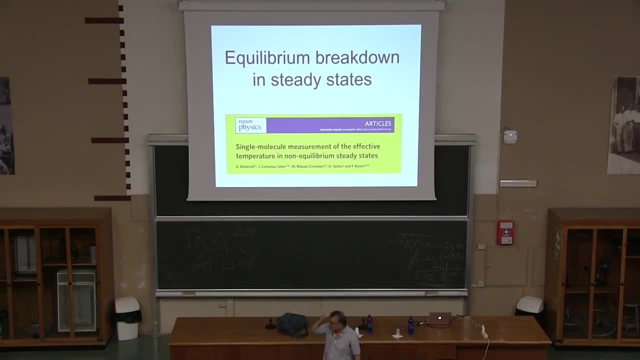 being so small. we had the resolution to see these things, of course, in equilibrium. I showed you that I can do it, so what I wanted to do it was, in the case of non-equilibrium, steady state for equilibrium, I did it for a molecule, so the question remains. 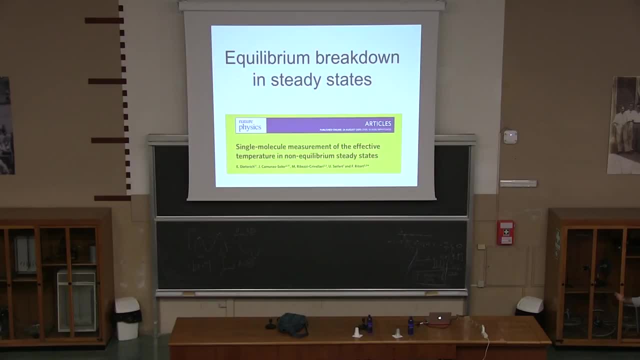 of what type of, let's say, fluctuation dissipation theorem or, if you want, quasi fluctuation dissipation theorem, because it's not satisfied? what type of relation do you find experimentally- and this is work done in collaboration with Udo Seifert and he had a student who came to Barcelona- 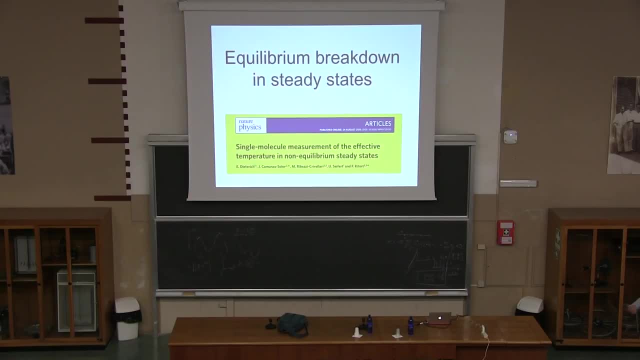 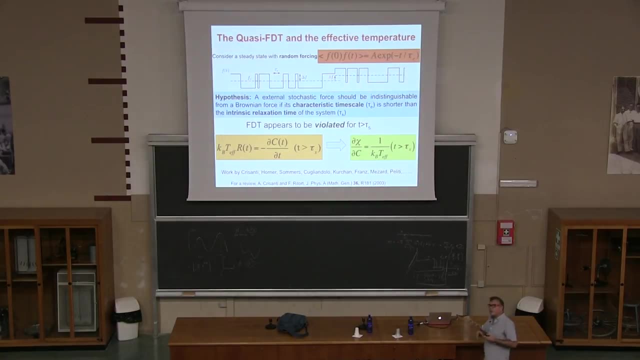 doing experiments and work and we somehow collaborated, doing theory and experiments together. so the easiest way I wanted to study this, the easiest way to implement non-equilibrium steady state, has been introduced by several people. Sergio Chiliberto actually did some of the experiments in the beginning. 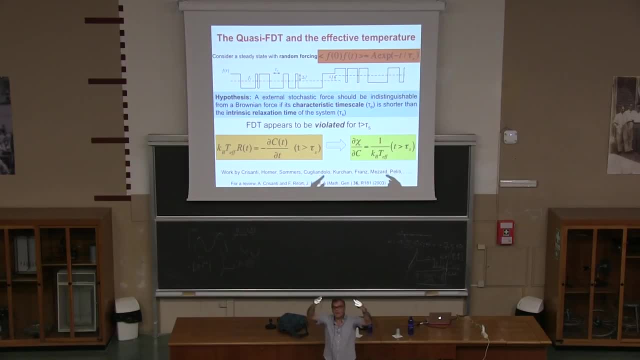 if I take an equilibrium system with a control parameter of the magnetic field and I start to oscillate the magnetic field not as a sine wave but stochastically, with a finite time, so exactly the control parameter changes dichotomically, as if it follows a dichotomic. 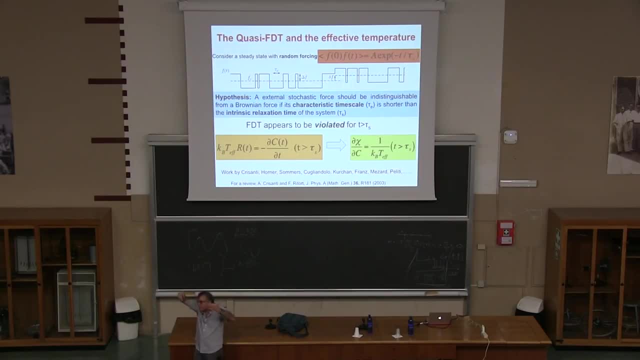 Orstein-Uhlenbeck process and of course I don't have a natural frequency there. I have a natural timescale for the correlation, but I don't have a natural, let's say, an oscillation. I don't have a frequency. I have a timescale, I don't have a frequency. 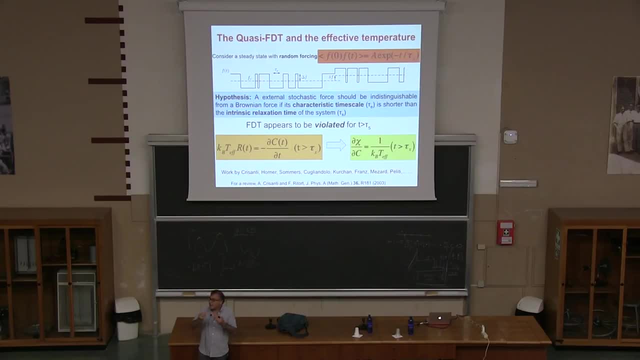 but still I am putting a timescale in my system and I am perturbing it. I am perturbing it because I am pumping energy with this oscillation, with this fluctuation. so I change dichotomically the signal between two values and then I put my system. 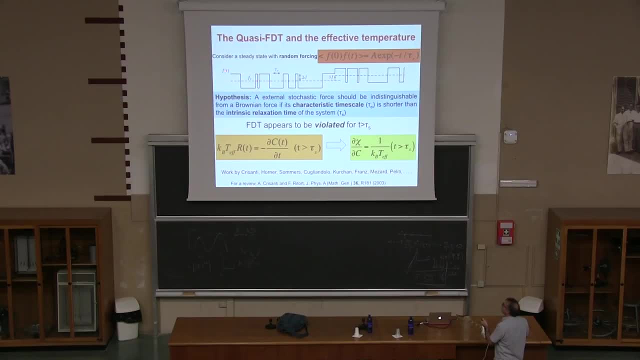 in a non-equilibrium steady state. there are two important values in this experiment. you will see, there is a force that fluctuates dichotomically with respect to a baseline, a centerline fc. so this is, let's say, the central force, and it fluctuates with an amplitude delta f. 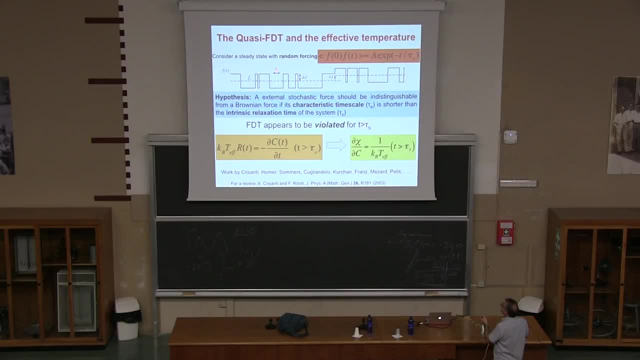 up and down, plus delta f, minus delta f, and has an intrinsic correlation time, tau e. so this force which drives the system to the nest, has this exponential decay form defined with this excitation timescale. and the idea- what we wanted to test was very simple, was the idea that we ask: 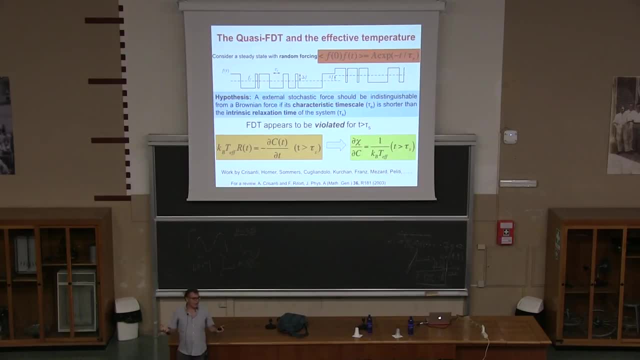 if the excitation timescale is much smaller of this random forcing than the intrinsic timescale of the system, then we thought, in principle, if this is true, the system should feel like if it is in equilibrium, but at another, higher temperature, because relaxing on timescales that are much bigger. 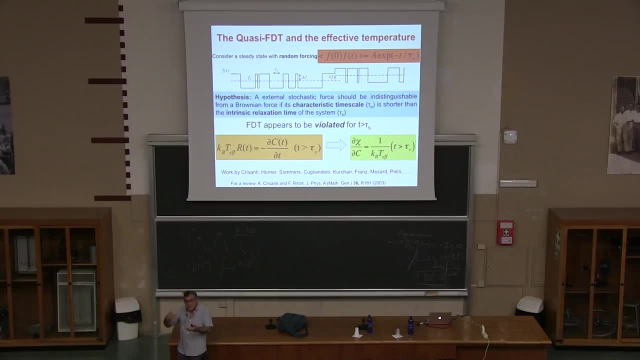 it cannot discriminate the external random forcing with intrinsic Brownian noise, because intrinsic Brownian noise also has this timescale, but it is picoseconds. conceptually should be more or less the same and, but however, if I look at timescales that are bigger than the intrinsic relaxation timescale, 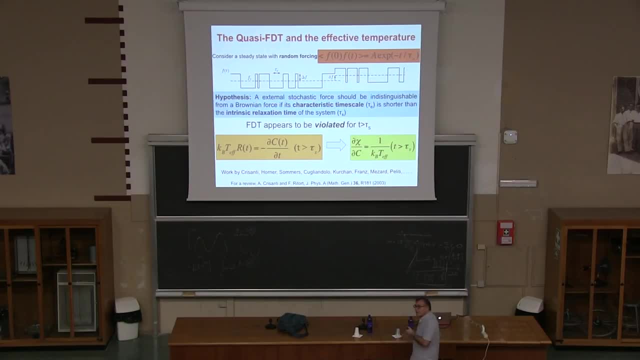 of the system, then I should have this form, and this form was introduced by many people. I list a few of them there that have contributed- but originally this was done by two seminal papers in 1993, I think, at the same time nearly, but the idea was there. 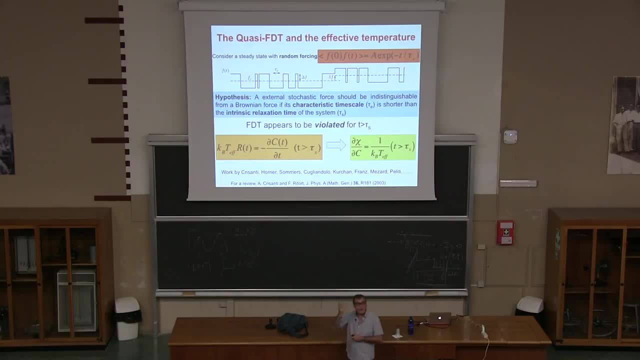 that there should be like an effective temperature, which is also called fluctuation dissipation ratio, four times bigger than this time TS. so somehow, after these times, you should feel this, this random forcing, and you should get a temperature that is different from the bath temperature. then we did experiments on this system. 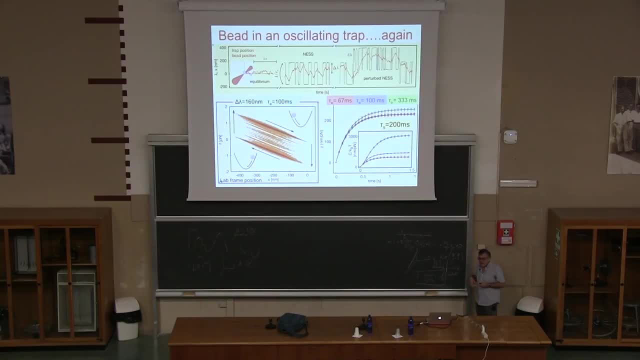 let me show you first. well, in equilibrium, of course, you get this thing. and for the bit in the oscillating trap, let me show you how the experiment works. you have now this bit in the optical trap and you have the atomic force which is changing. this is the black line. 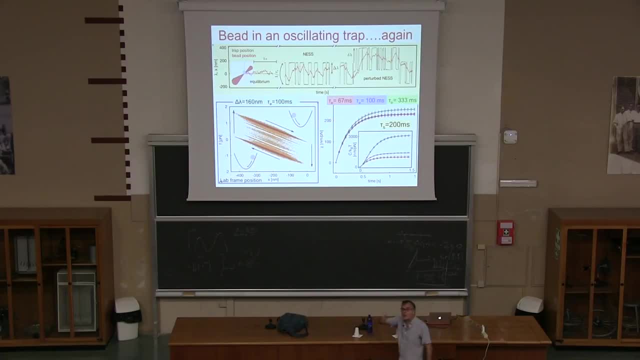 so the black line is the atomic force. so how can I control the force in this experiment? of course this is a bit in the harmonic potential. I cannot control the force because the force is determined by the viscous friction. I cannot control that. what I can do is 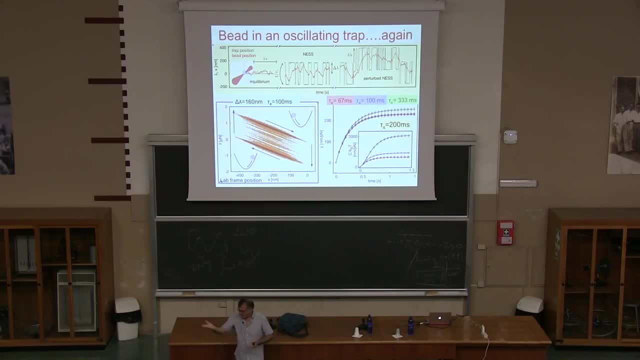 somehow mimic the force by moving the optical trap between two positions which are about, in this case, 160 nanometers, delta lambda. so plus 160 nanometers, plus 160 nanometers, minus 160 nanometers, and I can make the bit unhappy and crazy. moving between the two harmonic potentials. 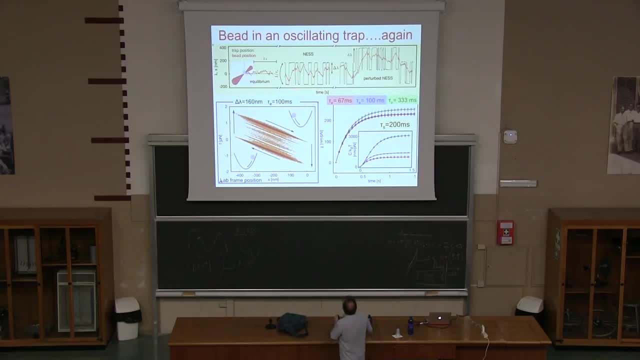 ok, that are shifted. now, what you see, if you do this experiment, is trajectory. ok, because when the position of the optical trap is here, up, the bit wants to go to the center of the trap. up, when the center of the optical trap goes down the trajectory of the 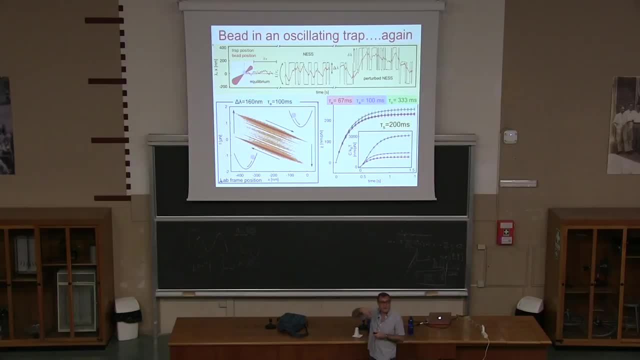 bit goes up, it wants to go here, but of course it cannot do it. it doesn't have enough time. and now this would give me- I could measure in this way- the correlation function, because I have just the signal. the red signal would give me the correlation function for the position. 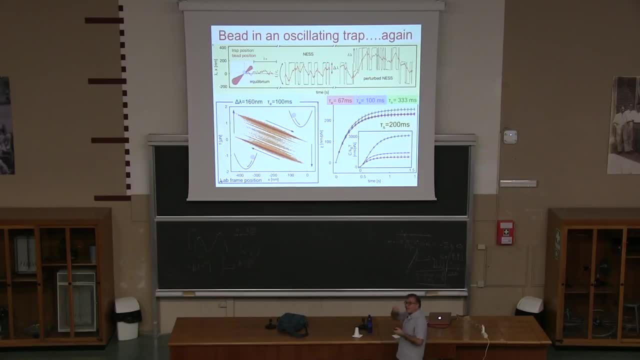 of the bit. at the same time, I can measure the response function in the non-equilibrium steady state by perturbing it. how I do it? so this oscillation, what I do is, at some point, instead of oscillating between A and B, I move A and B here. 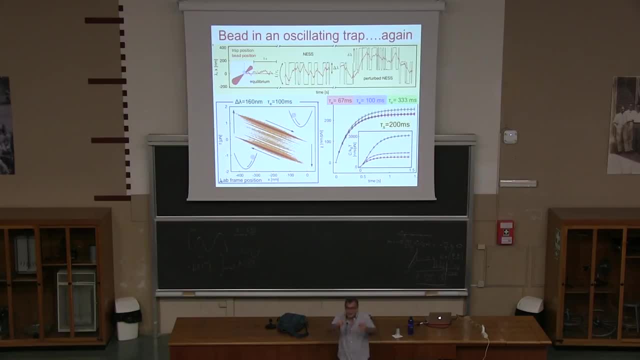 and oscillate between A and B, displaced. so there is a center of mass, let's say of the position of the optical trap, sudden jump to a new position and then the trajectory of the bit relaxes again to the new. so this region here gives me measurement of 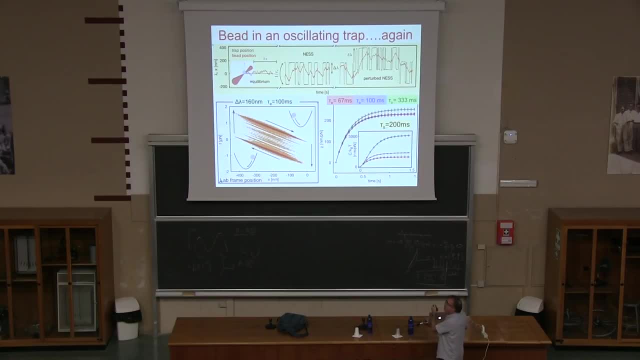 the susceptibility, because this is a jump step, it's not an impulse. ok, this stays forever. I saw, and so on. I come back to the original point. I repeat this many, many times and collect a lot of statistics. so here is what you see: a trajectory, typical realization. 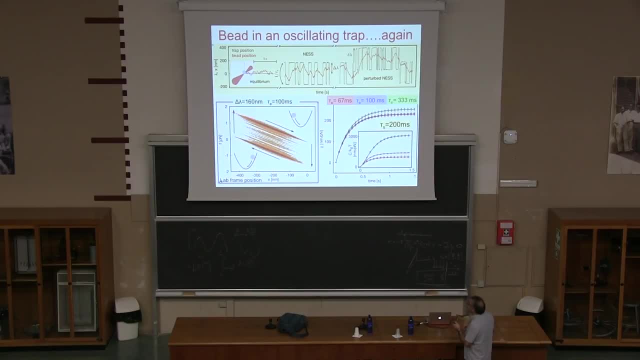 of the trajectory of the bit. of course you see that the bit, when it is in a position in a well, the bit oscillates between the center of the optical trap and because this is a hook and low, the force is proportional to the displacement. so if you fix the position of the trap, 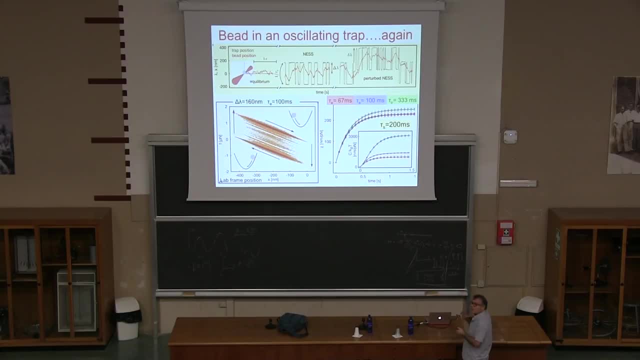 then the force follows this straight line, which corresponds to the stiffness of the optical trap. now, at some point, what you do is you move the position of the optical trap rightwards or leftwards. ok, it depends for you. for me, you move leftwards, the bit goes. 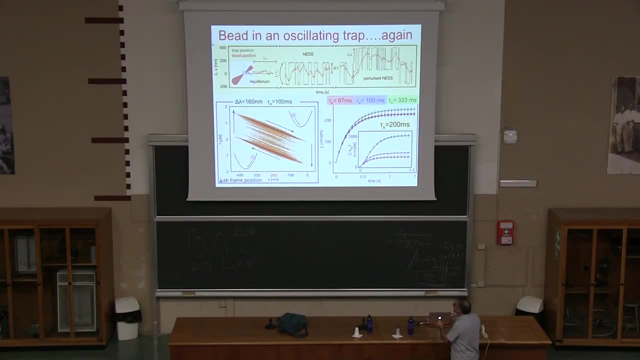 to the right immediately. but pay attention, this measurement is not x, is not the position of the bit respect to the center of the trap. this is x. is the lap frame position, is the position of the bit respect to the chamber. so, even if I move the optical trap, the position 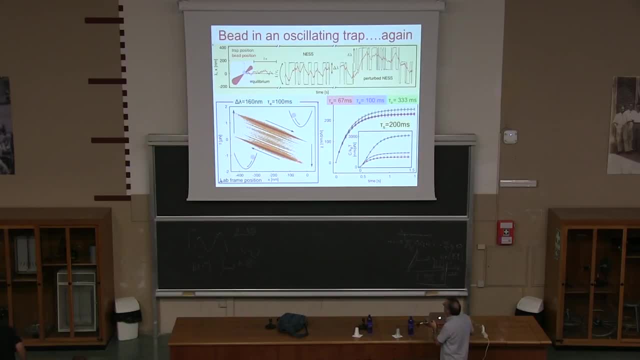 with respect to the lap is the same and therefore what happens is that this region doesn't change, but the force, because it goes to the other side of the well, changes ok, and it goes from positive force to negative force. so this change in force in Hookean force means that 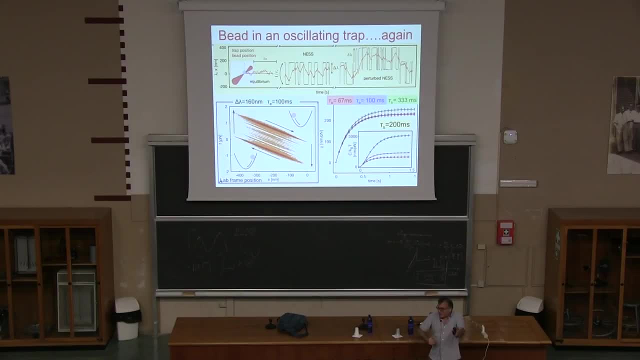 respect to the well is. but you know, I'm moving the optical trap, but in the lap frame the bit is in the same region, ok, and then you go up again by moving, by restoring the, the other side, and so on. now the important thing to understand is that 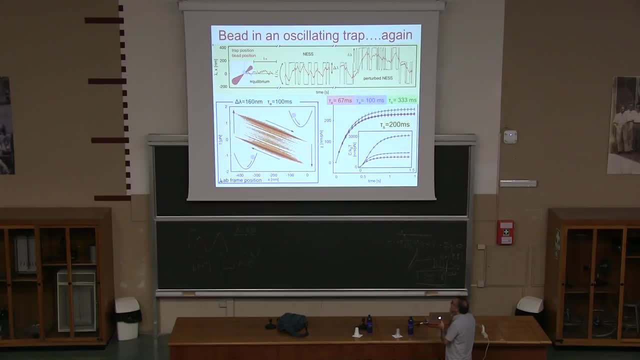 if I do these sort of trajectories, I can measure the area, the circulation of these lines in the two dimensional plane and therefore there is a net average area per unit time. so there is an entropy production. so if you were to do the experiment without doing this stochastic, 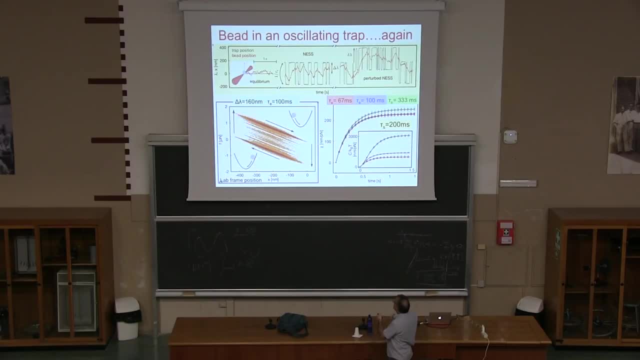 driving I would have also a very noisy signal just if I don't move the optical trap across one of these lines. but there would not be net circulation. so the actual entropy production is the area, the average area per unit time or per cycle in these sort of plots. so whenever 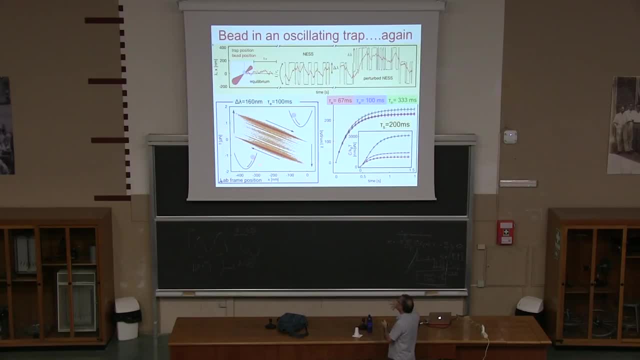 you make a representation of one force or one variable, like an observable, magnetization or the position or whatever, and its canonical conjugate its corresponding force. if you make a representation of trajectories and you look there is a mean area per unit time. this means that you have an. 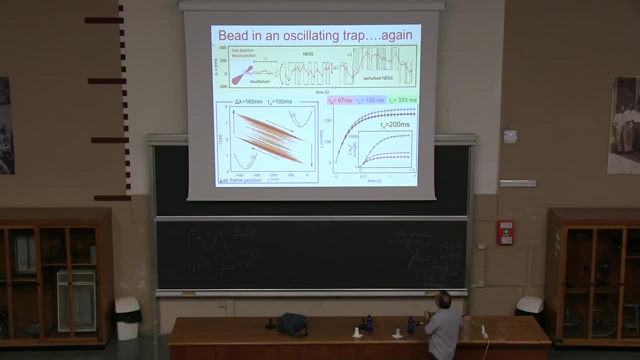 unequilibrium state because you have a net entropy production. so here we measure the correlation function, we measure the susceptibility for different excitation times. so the average excitation time in this signal could go from a low value, 67 milliseconds, to 330 milliseconds. so the basic relaxation time of the bit. 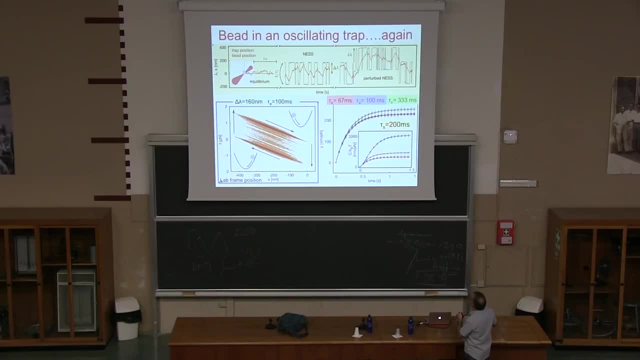 in the optical trap, which is due to friction and due to the stiffness of the optical trap, is 200 milliseconds, so it is in between these two regimes. now it turns out that the susceptibility you can prove, you can make analytical calculations on this model and should not depend 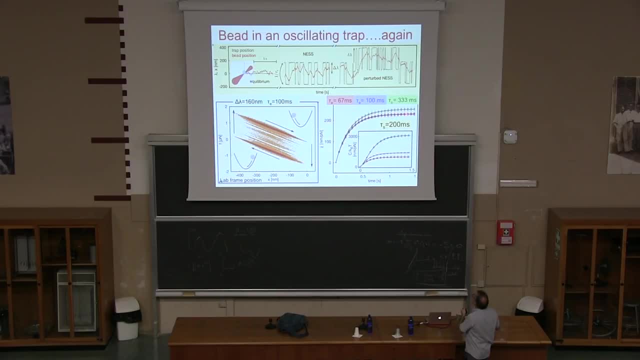 on any of these parameters, and here you see a slight difference. but this is experimental error, because we know analytically that it should not be like that. but the correlation function should depend a lot on tau e, so even if all these curves have the same intrinsic relaxation time, 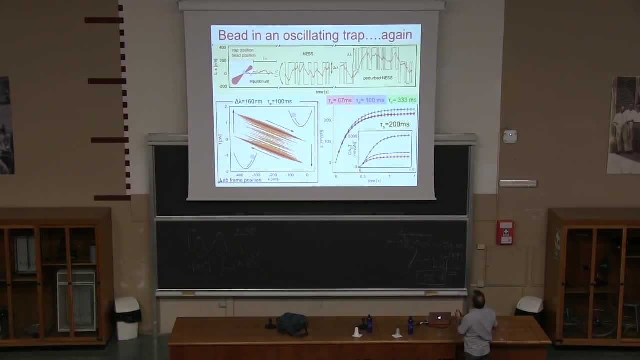 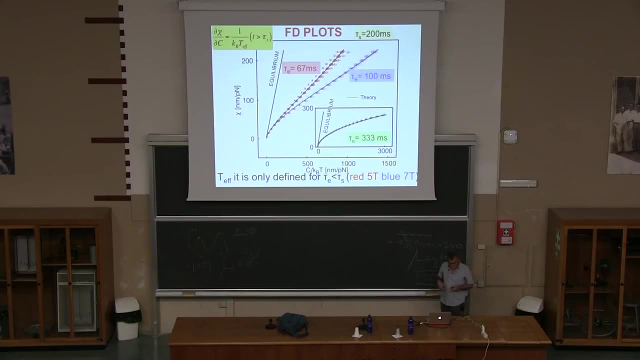 because it is the property of the optical trap. here is the property of the random switching between the two positions of the optical trap. there is a change in the correlation function and now you can build the FD plots. and we were surprised that, even for the bit in the optical trap. 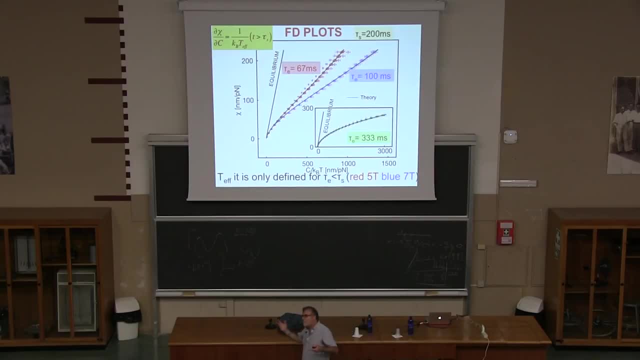 that everyone has studied in the framework of of non-equilibrium, let's say experiments. the microsphere and optical trap is a very much experimental realization of a very simple Langevin model. this calculation had never been done by anyone. I don't have the time to show you the details. 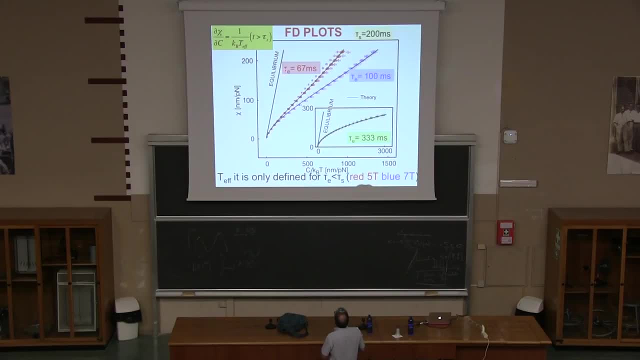 but basically we demonstrated that when this time, tau e, is less than the excitation time, the intrinsic relaxation time, when the excitation time was smaller than the intrinsic relaxation time, this idea of the excitation of the random forcing is true and you developed an effective tamper. 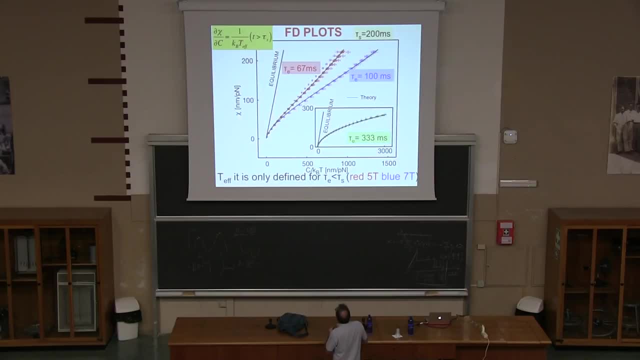 so you develop in key over C. you develop a line, so you initially start tangent to the equilibrium. so slope equal to 1, if you want, here in this plot, which is this equilibrium line, but you depart immediately and only for times that are bigger than the time tau s. 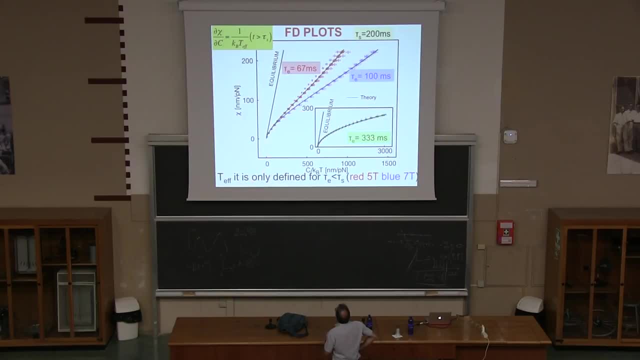 200 ms, you start to see these straight lines. so here the effective temperature would be: for the red, which is 67 ms, it's 5 times temperature. for the blue, it's 7 times temperature. so this is actually high because temperature is 300 K. 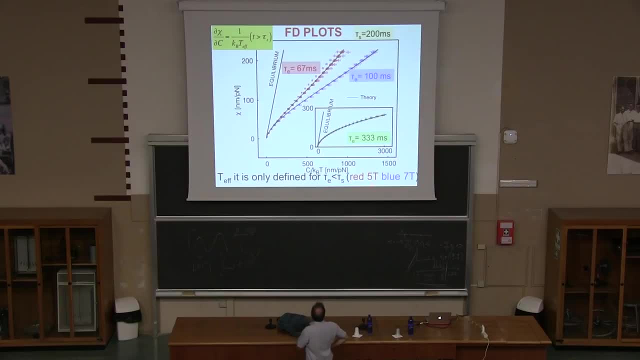 so this is 1500 K and the other case is about 2000 K. now, if you go to a condition in which the excitation time is longer than the intrinsic relaxation time, there should not be, this idea should not hold. and actually what you find and you can demonstrate analytically, 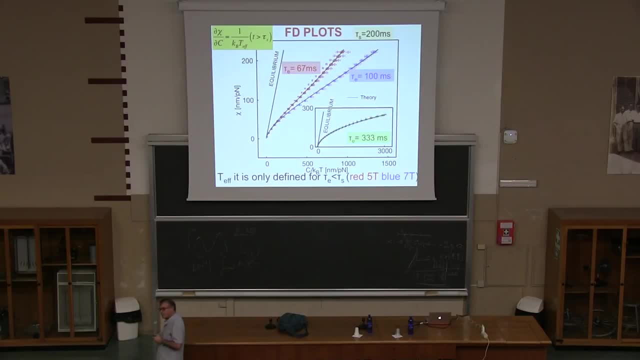 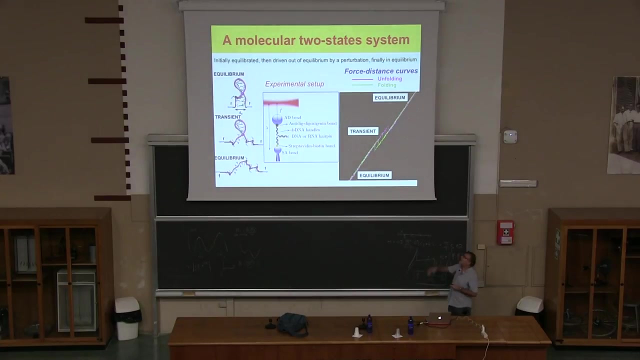 is that there is no straight line behavior. everything curves always. so this is an experimental realization of a simple model. and then, to make the story on this part of my talk relatively short, we went to a more complex system and we investigated a molecular two-state system, which is a molecule that holds 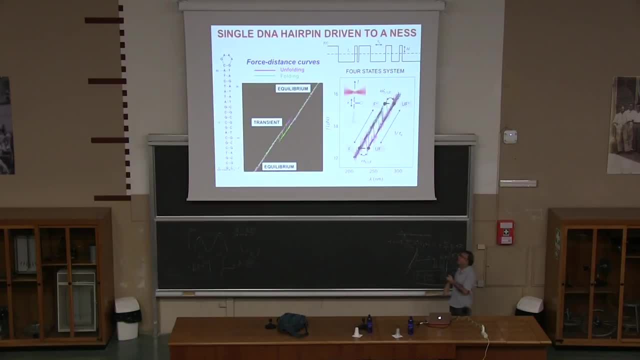 between two states with force. I showed you before the experiment and here I can do the same. I can switch the force ecotomically and I can see in this condition whether there is entropy production, whether I am out of equilibrium, and I can plot the force as a function. 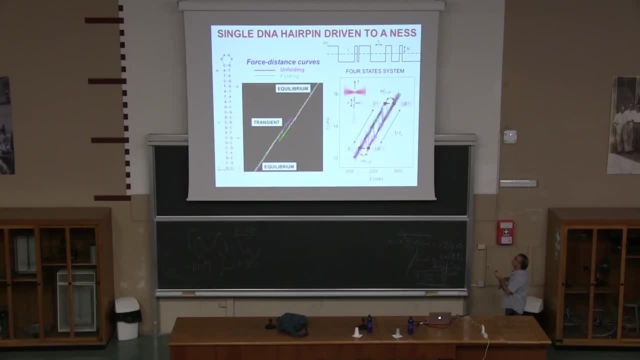 of the position of the optical trap and again the molecule. suppose that the molecule is at a given force and then if the molecule spontaneously unfolds, the force drops. if the molecule spontaneously falls, it goes up. but also I can move the position of the optical trap and by moving the position of the optical trap, 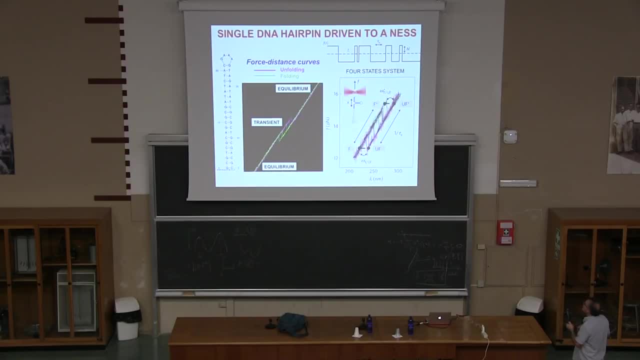 I can make transitions from here to there. so I have, let's say, four types of states at a given position of the optical trap, like this one. I have two states of force folded and unfolded at the other position of the optical trap, more tensed, for example. 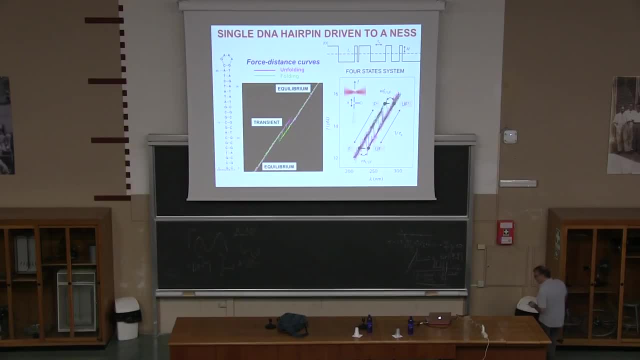 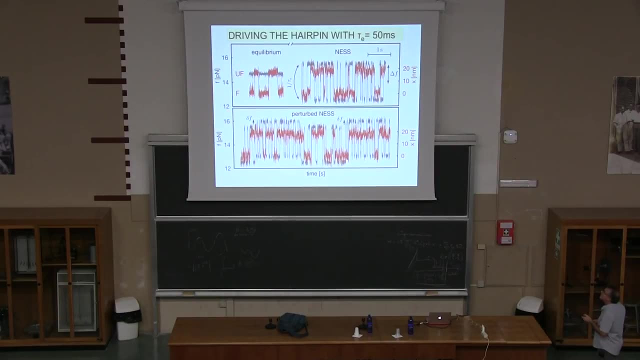 I have two other states, I have four states and these four states are represented by these four points and I have finite circulation. so I have entropy production and I can take my trajectories experimentally measured in equilibrium. then I have this grey line is the position of the optical trap. 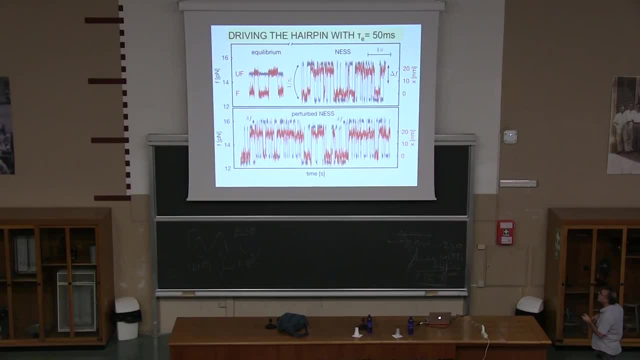 which actually here what I am controlling for a long time. so this is basically the force imposed on the molecule with one kilohertz frequency. so I keep a condition which is constant: the molecule hops between two states and then I produce my nest by switching the force between two values. 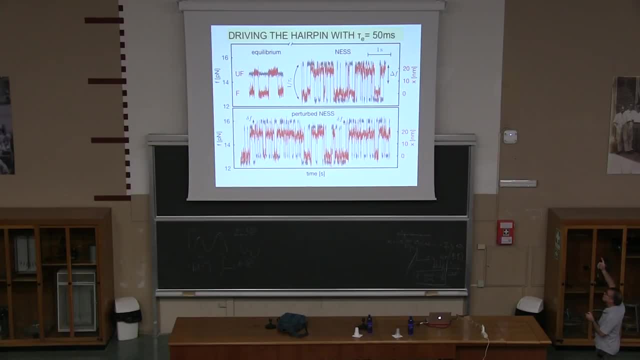 let's say 16 piconewtons and 14 piconewtons, delta F is 1 piconewton and the center is 15. switch back and forth with this stochastic switching which has an average time, in this case, of 50 milliseconds. 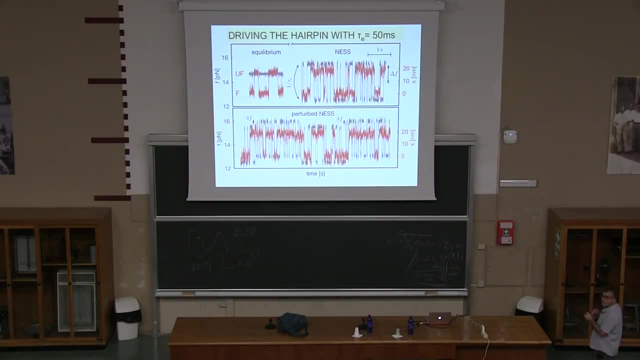 so the response in the hopping between the two states is also in there in this red signal. and then I can do the experiment where I perturb the non-equilibrium state by shifting the 15 average piconewtons to another value and then I measure how these trajectories 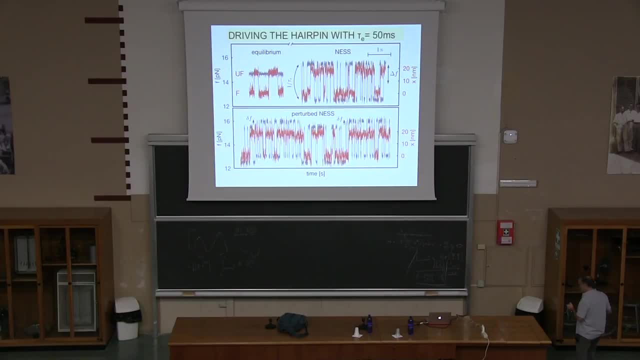 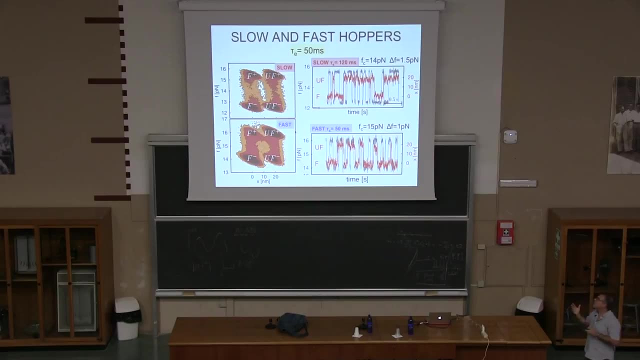 when I do this change, these red trajectories change. then we started. we always wanted to compare with this intrinsic relaxation time with respect to the excitation time. here is 50 milliseconds and we studied two molecules, one molecule which is slow compared to T, so 120 milliseconds. 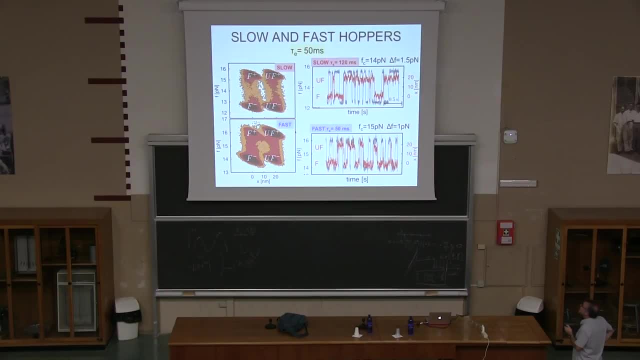 meaning that the switching is faster than the hopping of the molecule. and another case, fast, where the switching is comparable. in this case is comparable. moving in these timescales is difficult because you have to find conditions where one herpin has a given timescale beyond or above. 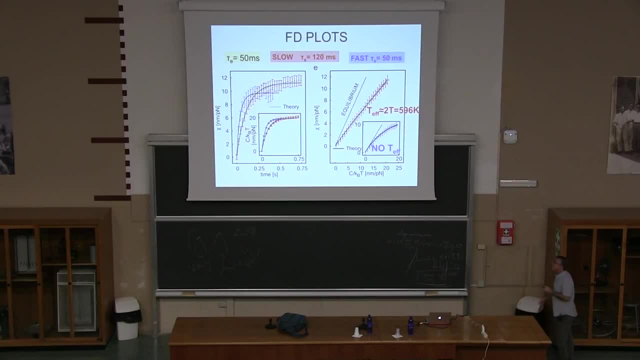 the structures accordingly. anyway, the important thing is that when you do the measurements of the correlation and the response and the integrated response, you find this. we developed also a theory for the forested model. that works pretty well, but then you see, for the system in which you had. 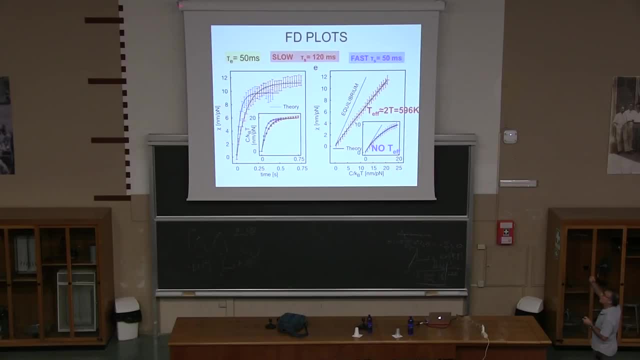 the slow herpin, the system in which the random switching force can be considered to be an aided Brownian motion. then we see a straight line with an effective temperature, otherwise the room temperature. but in the case of the fast, we see the curvature and there is no effective temperature. 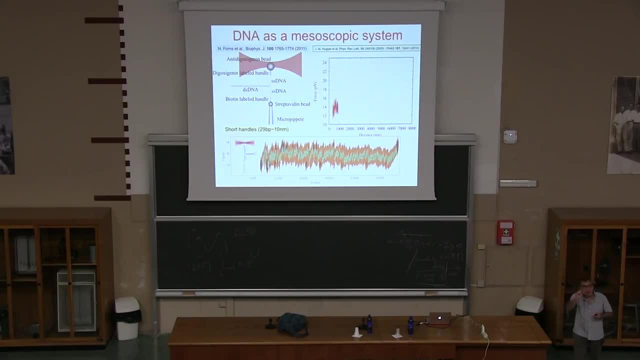 and you can go even farther. you can go from the small to the mesoscopic and you can imagine that you don't take just a herpin of 20 base pairs like in the previous case. it's short, so this is 20 nanometers in opening. 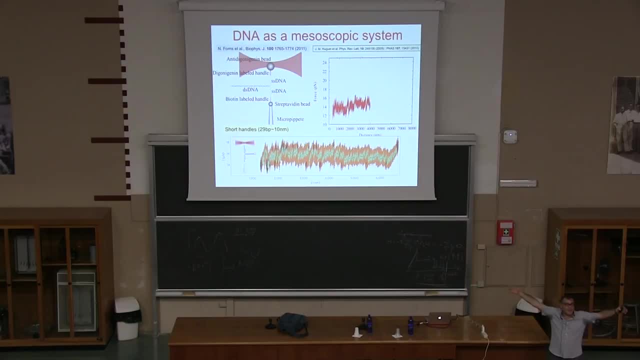 you can take a molecule of 6,000 base pairs that opens like 7 microns, so it's a really big molecule. so here I am approaching the macroscopic limit and you want to see how you go from the small molecular nanoscale to the much larger scale. 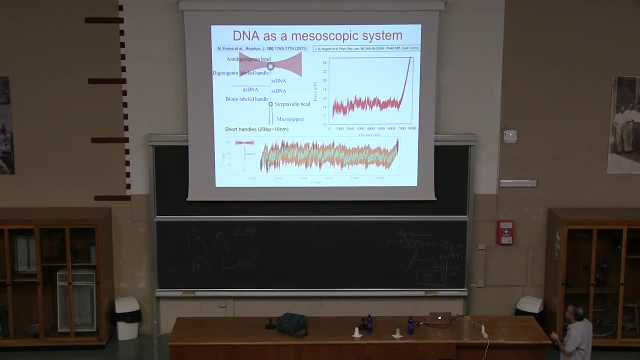 micron scale. this is the molecule, how it would open sequentially from the beginning of the stem to the end. this is 7,000 base pairs. and now what I do is again the same thing. I do: a stochastic forcing a random switching of the force between two values. 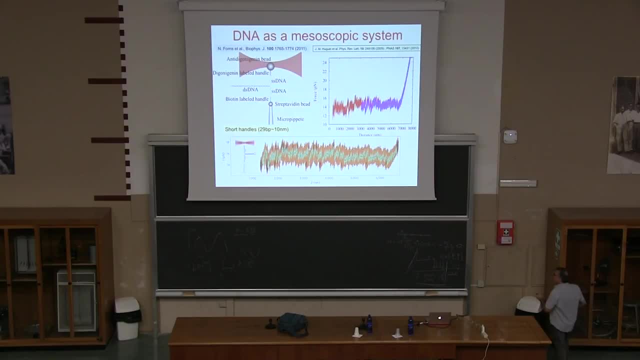 and then I produce all this sort of noise and structure. so here is the tail of a trajectory. um well, this just wanted to show you that the molecule unzips and rezips reversibly. this is something very nice, because it shows you at the molecular level. 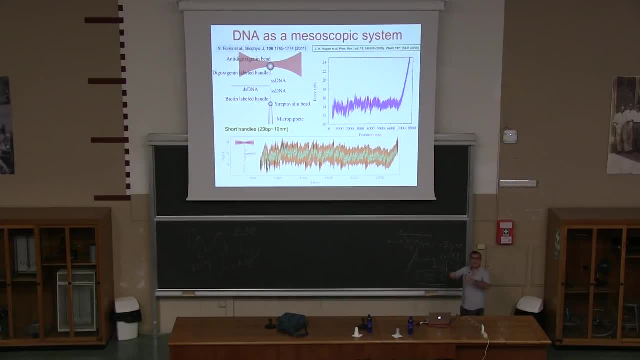 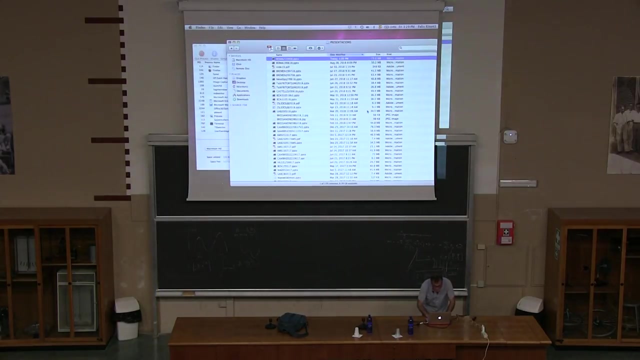 you can have reversible behavior, even if it is 7 microns long. so it's like if you take a piece of chalk, you break it, you connect it and then you reform it again. so that's very interesting. and then, oh sorry, what happened here? ok, I think I put too much weight. 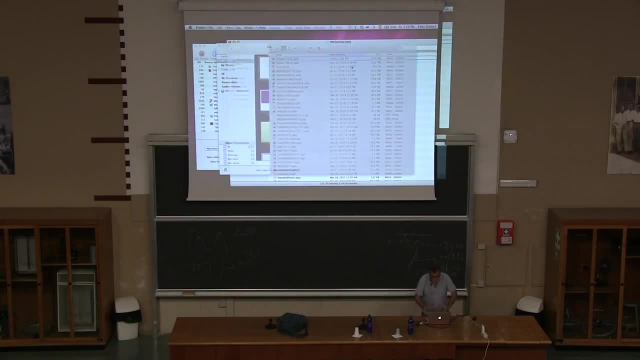 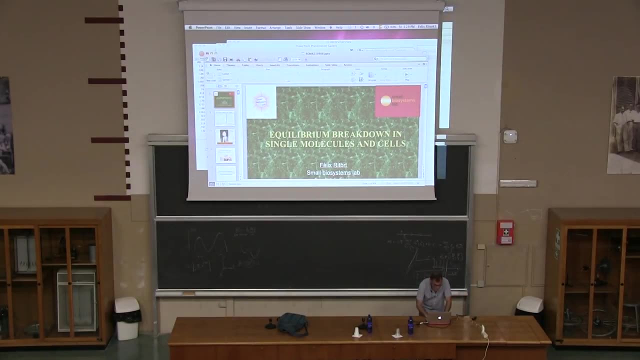 in my presentation, too many slides. but what it shows you is that when you do the experiment, in that case it seems- also because you are in the condition- that the excitatory time and the intrinsic relaxation time are very well separated, and in this case, um, I think here, 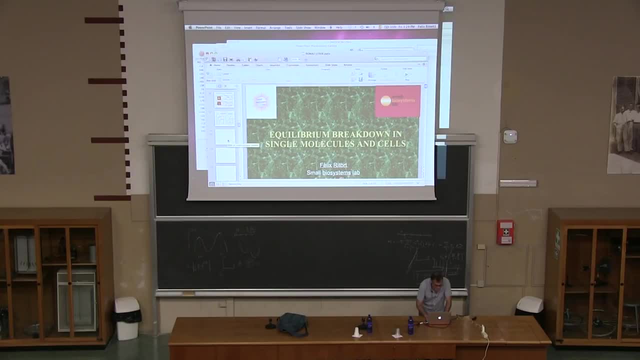 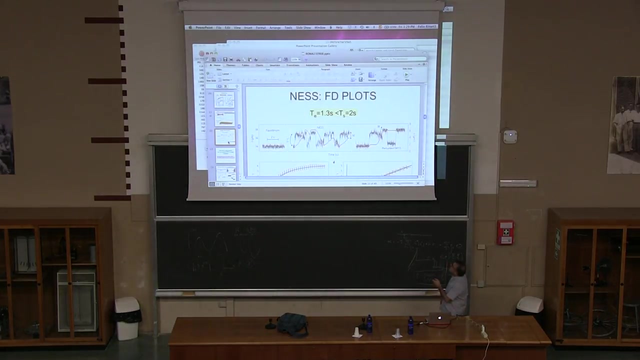 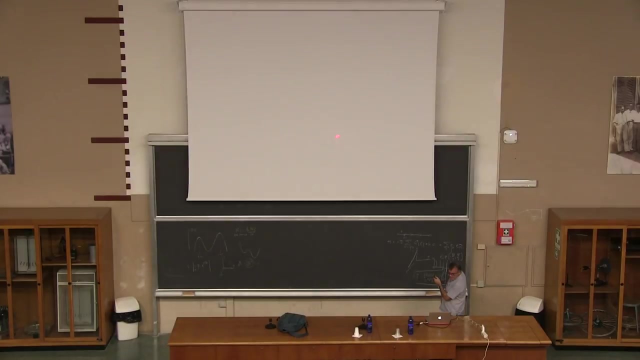 is the figure. the excitation time was 2 milliseconds and the intrinsic relaxation time is bigger. let me see if this goes here. ok, here you see the trajectory. so the intrinsic, uh, so the excitatory time is 1.3, ok, 1.3 seconds. 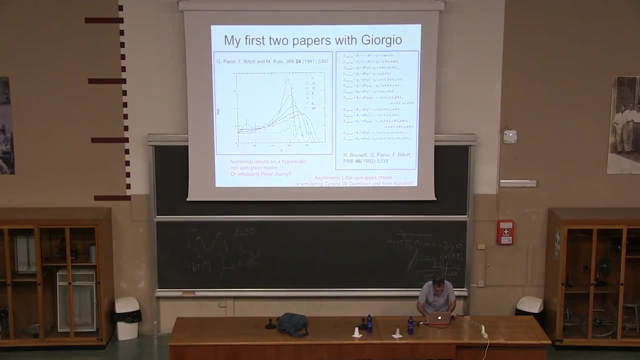 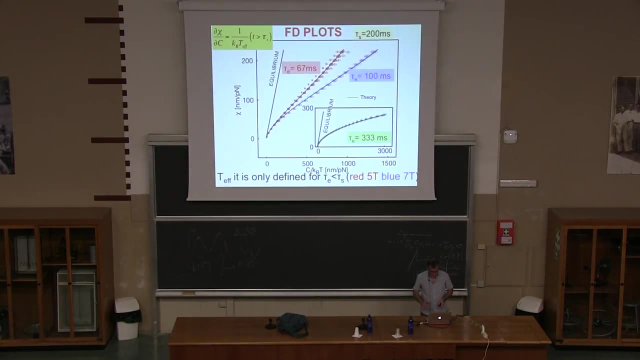 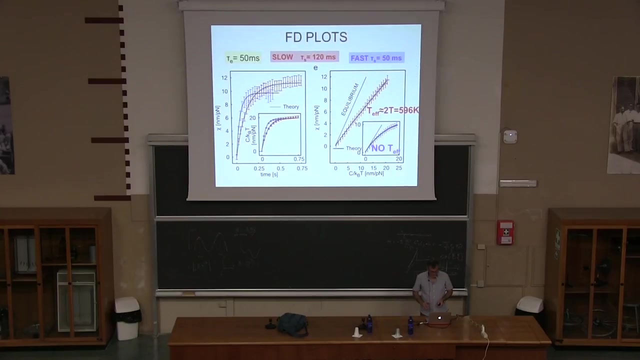 ok, so let me just, uh, let me just- I don't know what's going on. it worked, I mean, I tried it. ok, so it's 1.3 seconds excitatory time and the intrinsic relaxation time is 2 seconds. so again, you are in this condition. 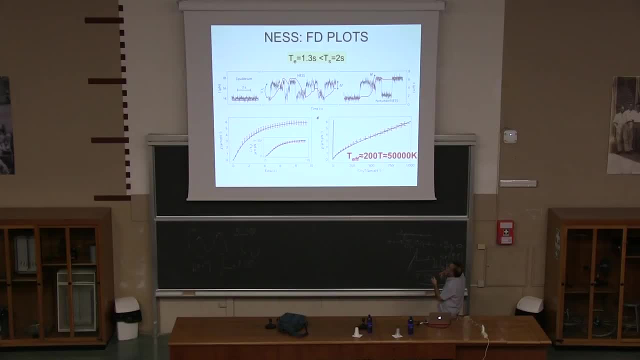 and then you can generate the same thing- FD plot- with effective temperature which is 200 times so when things got bigger. so this means that these effective temperatures can be actually very, very large. so let me just make a mention that this thing that we have done, non-equilibrium steady states. 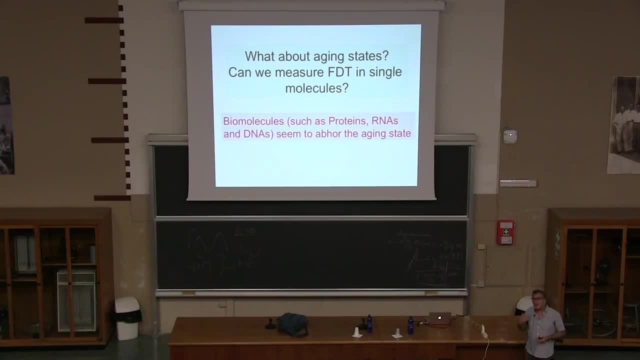 we would like to do for aging states. so it turns out that single molecules do not want to age. either they fold or they misfold, but you never see them aging to the non-equilibrium state. it's very hard, and this is something which is very common. 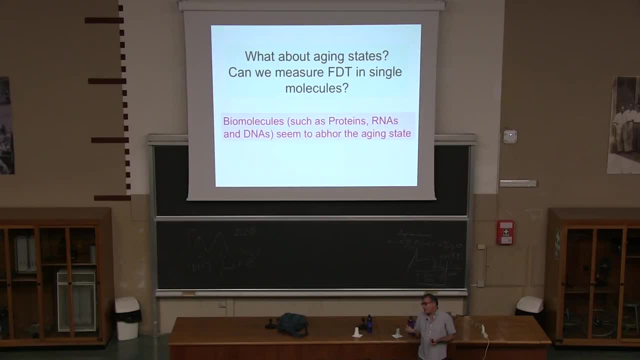 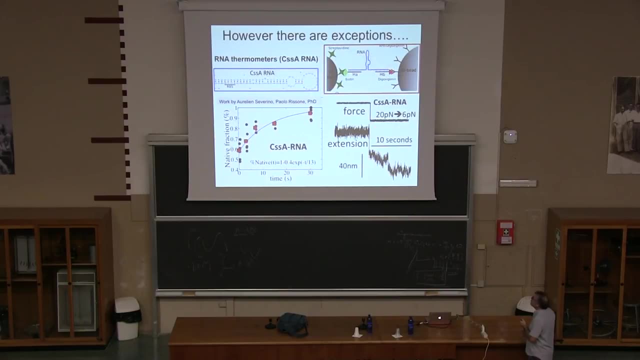 and it may have a biological meaning. this means that molecules have to be functional, so they have to either fold or misfold. you cannot have them slowly relaxing. but there may be exceptions, and one exception is something we are doing in my lab. I show you here this work done by Aureliano Severino. 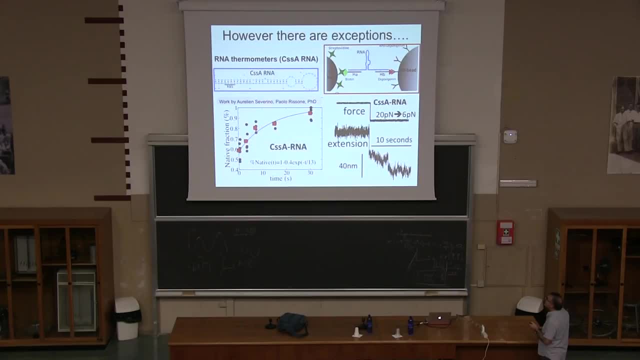 which is a very talented student in my lab, who is in Switzerland, and Paolo Rizzoni, who is working also in the lab, working on RNA, and he is a student of Georgia. he is here in Barcelona since one year and this molecule is an RNA that has a complicated 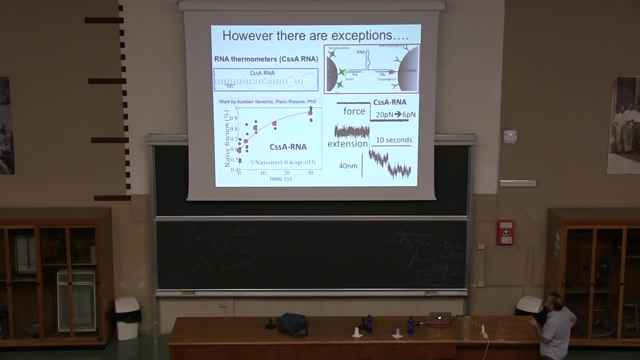 structure because it has these non-complementary base pairs. it has bulges. it is what is called now an RNA thermometer. it has been discovered that many illnesses like, for example, meningitis, occur. so meningitis basically is an illness by which, when you get fever, you activate. 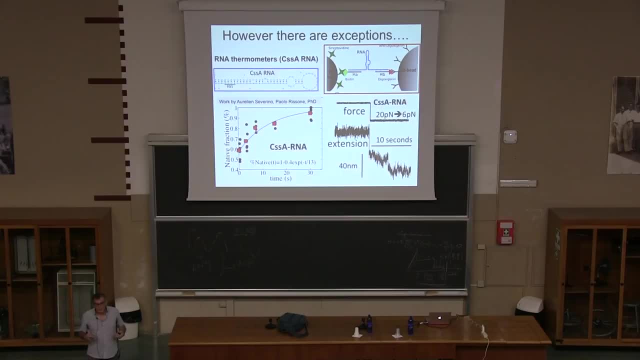 you don't deactivate, you activate the whole response of the virus. and this is because this virus, so it's supposed that when you increase the temperature of the body it should kill the bacteria. but something different happens. this virus, or these bacterias, when they change temperature, they activate a response inside. 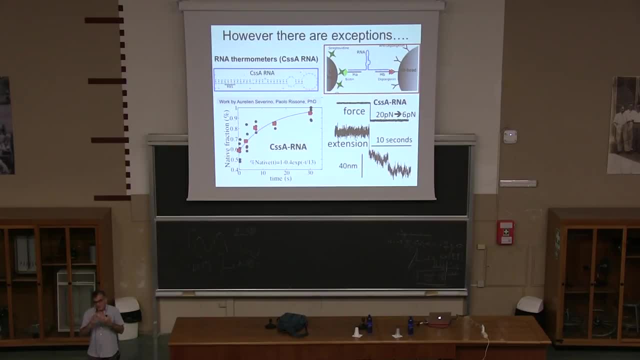 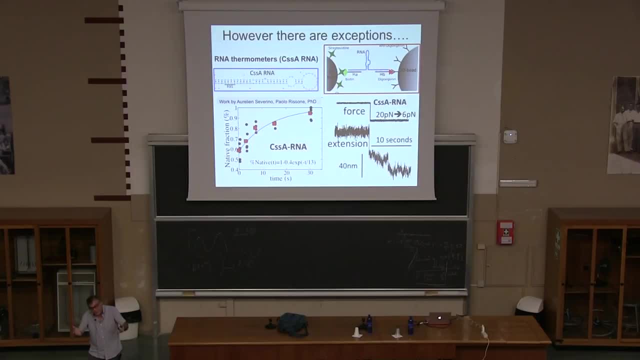 and then it starts to express in some protein that at room temperature 37 Celsius was not produced. so you go above 40, they start to produce and then, even if your body increases temperature, the bacteria become more resistant because they start to have new molecules that can fight. 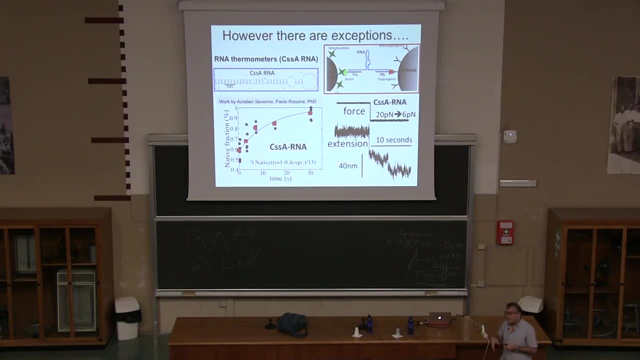 increase in temperature, they are more aggressive and they kill you, and meningitis is one of these. and this is this case of this molecule that has a transition to another conformation and because it has another conformation, it has the possibility to have other states, and what we see is 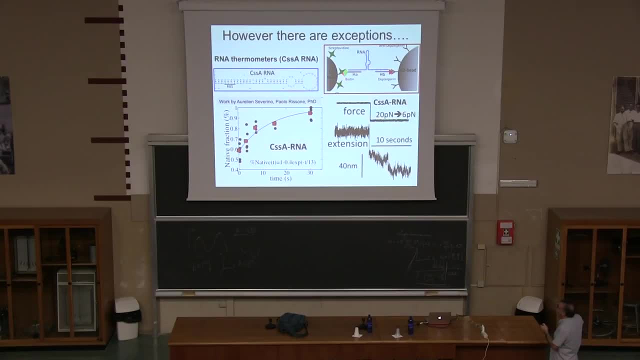 that when we study this molecule and we quench from an unfolded state to the native state, we see that the native state is reached, okay, but only after some time, and the fraction of native molecules, as a function of time, follows an exponential behavior with a time scale. this is seconds. 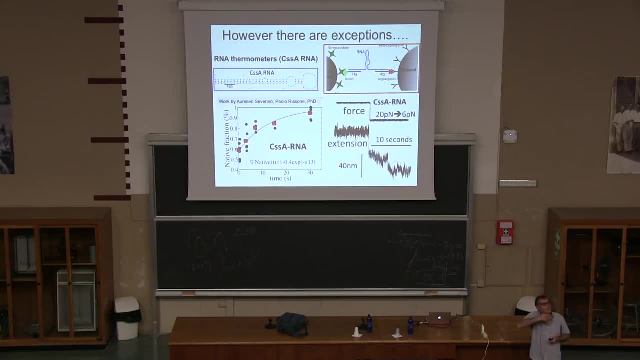 time in seconds of 13 seconds. so this molecule falls in 13 seconds. but 13 seconds for a molecule is huge, because molecules fall in microseconds. say, oh, this is not the age of the universe, like in a spin glass, but still 13 seconds. so we have to. 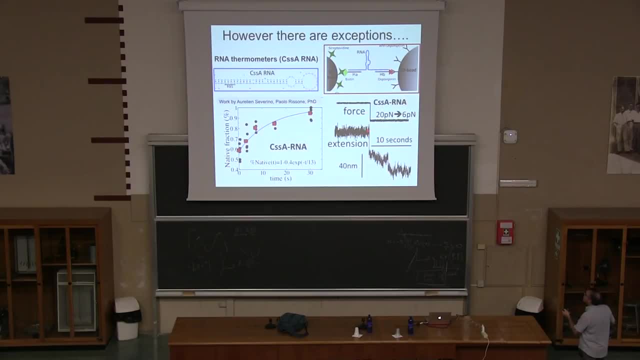 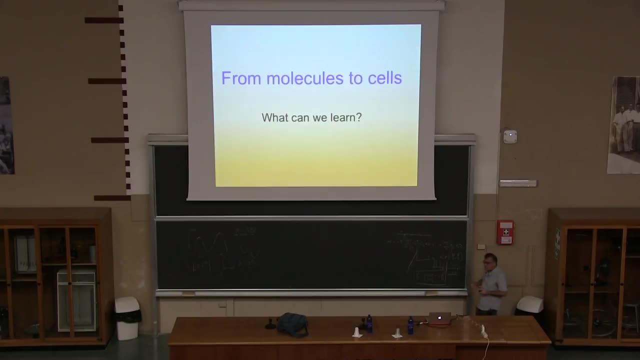 study aging non-relaxational properties in this time scale. so this is a curve, a typical trace. when you switch the force, the extension shows this low relaxation. this we are studying now. I will finish my talk because I think I have 5 minutes left already. so just mentioning that, the same things. 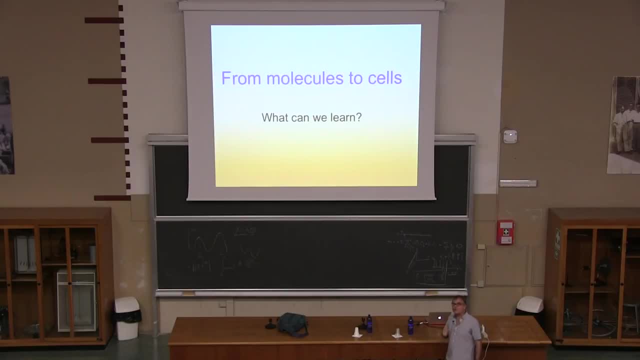 so you see, molecules are very interesting, but cells are even more interesting, and one thing we wanted to answer is whether physical aging and biological aging are the same or not. so the fact that, of course, cells age and they have mechanisms for that and they die, also red blood cells, which are 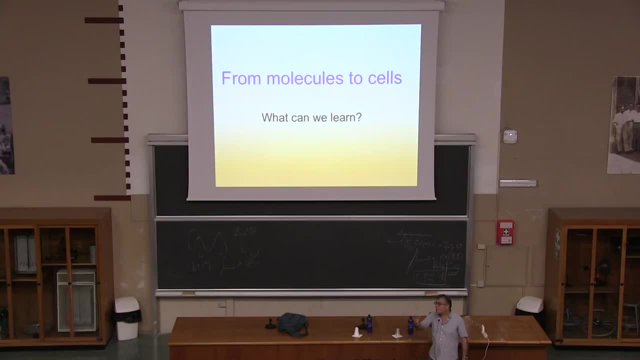 non-living cells. they have an average lifetime of one month, so they go through the spleen many times until some time they change their structural properties and some macrophages in the spleen see that they have changed it, and then they remove it and then new red blood cells are secreted. 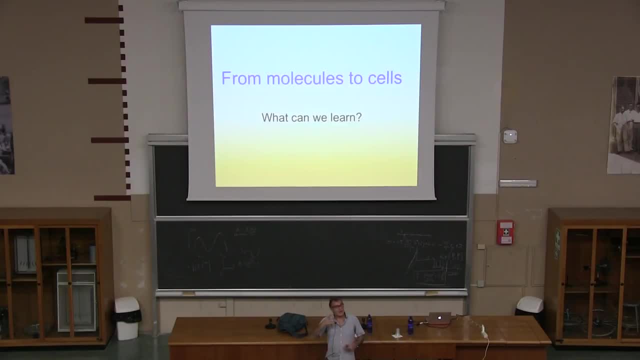 in the bone marrow and then you start the cycle again. so red blood cells, even if they are not living cells, they have an age. ok, and the question is whether we could investigate whether discriminate biological aging from physical aging. to make the story very short, you can do the same experiment. 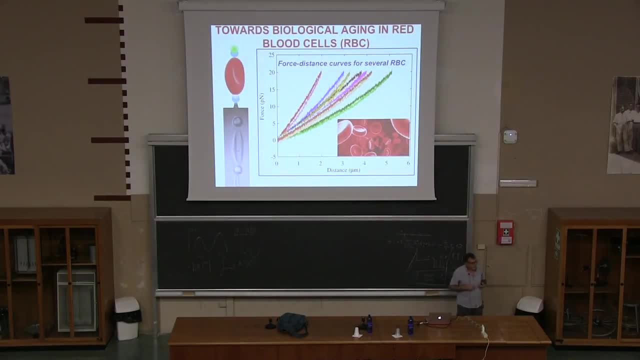 when pulling molecules, by deforming the red blood cell, and this has turned out to be a very beautiful experiment, because what you can do is exactly the same as for the molecules: you can measure the mechanical response of the cell across pulling, stretching and releasing cycles. these are examples of different red blood. 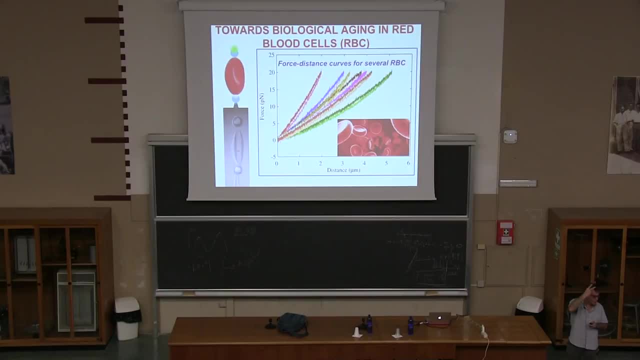 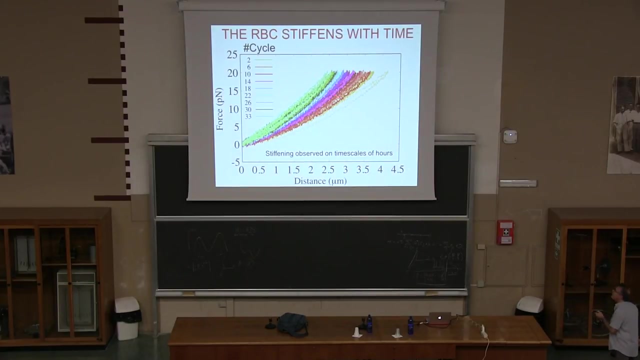 cells just curves, so there is strong heterogeneity. there are not two red blood cells identical, although there are two single molecules identical, because molecules have not the variability through sequence that a complex object like this may have. but we discovered something nice, which has been also reported by other people recently. 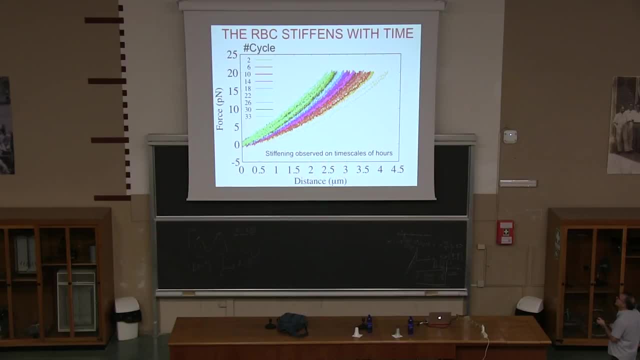 that is, if you force you cyclically repeat the pulling experiment over the same molecule many, many times, ok, for the same force, up to 20 piconewtons, the molecule shortens. the molecule, sorry, the cell shortens, so it becomes more hard to deform, so there is a stiffening of 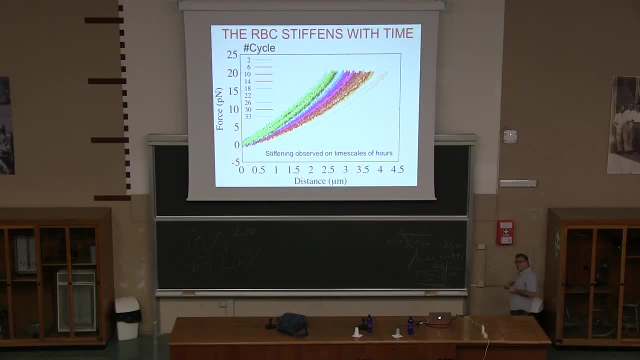 certain type scales of hours, and we don't know if this is biological aging or not, but certainly there is a time dependent phenomenon. so, on top of the non equilibrium steady state, because this is hydrolyzing glucose all the time, hydrolyzing glucose all the time. 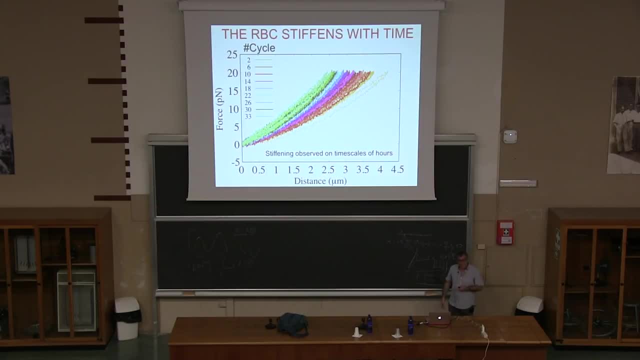 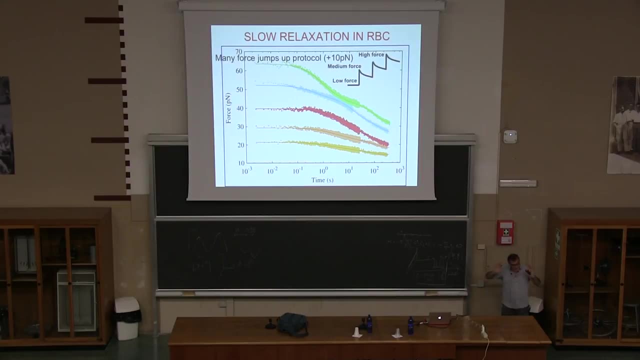 in the glycolysis process. at the same time, it is stiffening. then we took these cells and we did a lot of, a lot of non equilibrium experiments. ok, and just to make the story short, we start to play with this as if it were a magnetic 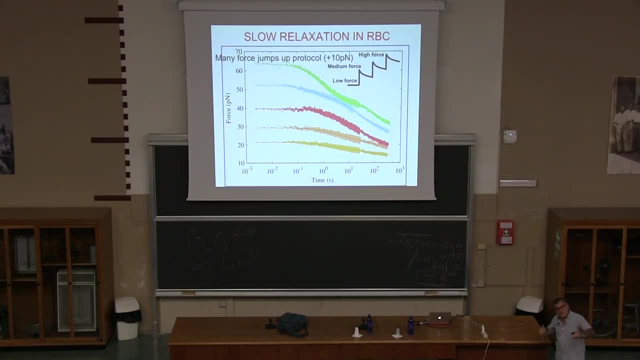 system putting a magnetic field using the force, then you bounce see how it relax. this is what you see, for example, if you do many. force jumps up in a protocol. so you start from 10 piconewtons and you switch up to 20 piconewtons. 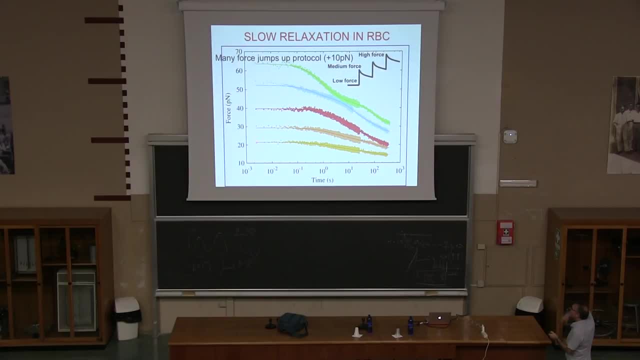 and you see, and you keep then the force out. I mean you just leave the red blood cell and the force decreases slowly. then you go from 20 to 30 and you see a new relaxation of the force from 30 to 40. you do a step, 10 by 10. 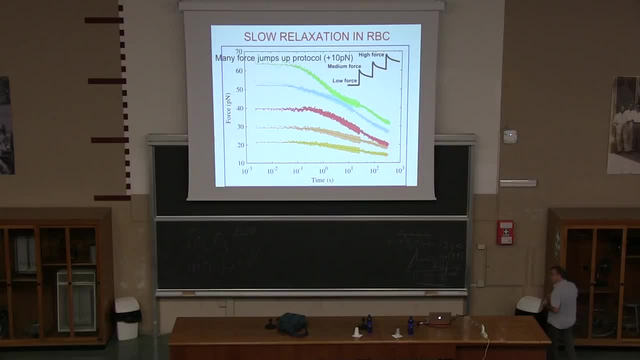 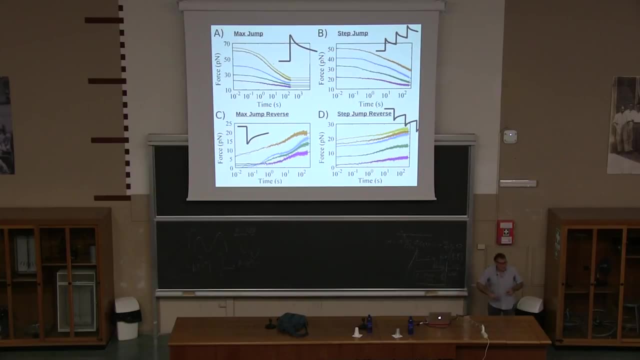 and you have this very interesting relaxational behavior, which is very complex. by the way, this is fitted to three exponentials and, to make the story short, we did many experiments: switching up, switching down, switching right, switching left, everything you can do- deforming, many types of deformation. 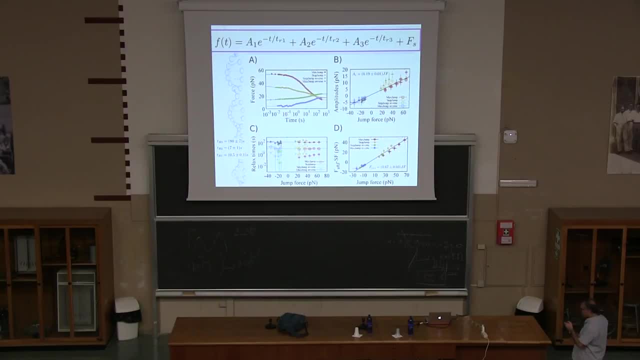 protocols and we always saw these three timescales so we could fit our curves with three exponentials, but at a stationary value. the interesting thing is that all the experiments we did, all the protocols, demonstrated that the relaxation time- there are three intrinsic timescales in the red blood cell that are independent of how you deform. 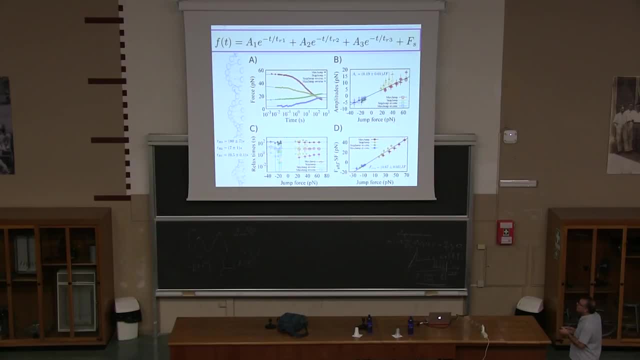 which is one second. let's say 10 seconds or 100 seconds. these are the timescales we could reach. they are very well defined. this is a very stable system. it's like you don't believe when you see it in the experiment. this is a possible red blood cell. 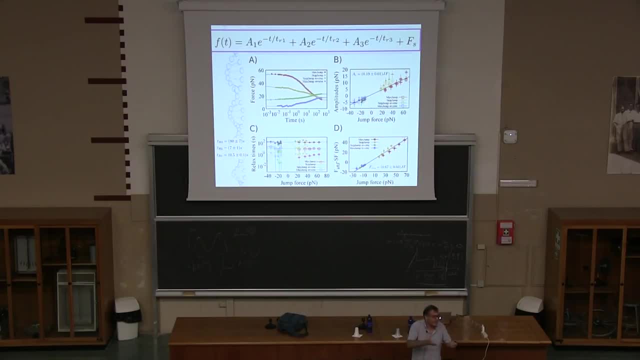 I have not found any soft matter system- artificial, let's say synthetic- that shows this behavior. and then, not only that, you discovered that even if you deform by 50% of the length, the linear response theory works. so the amplitudes are proportional perfectly to the changing force. 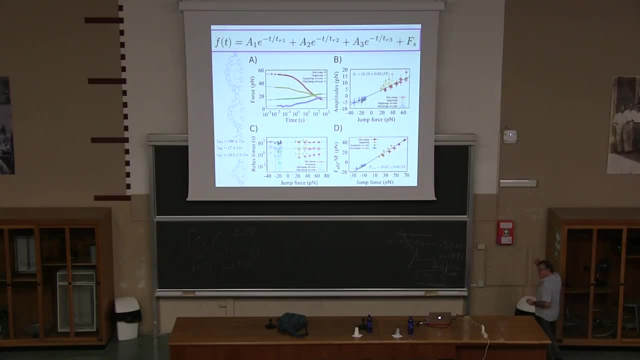 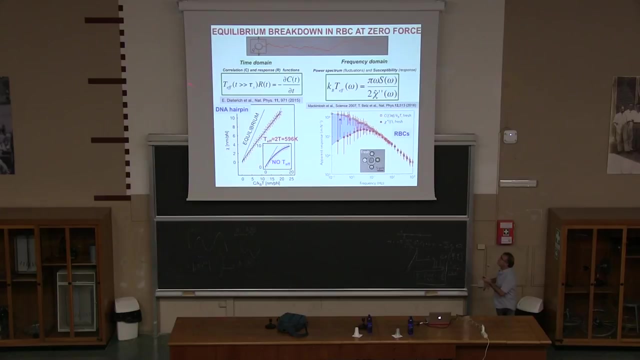 you have linear responses everywhere, and this is not only in my experiments, also in the experiments by in Amsterdam with acoustic force spectroscopy. he deforms up to hundreds of piconewtons with acoustic forces and see this linear behavior. this astonishes me how much you can go. 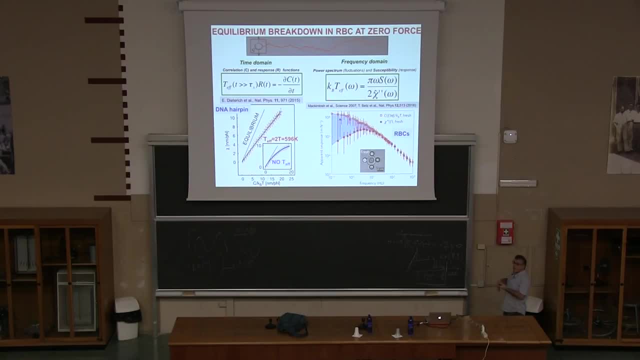 of course, in these systems you could ask the same question: whether there is equilibrium breakdown. of course there will be. this is something we are investigating now. I just wanted to tell you this has been done for cells, for red blood cells, actually by Timovets, but at zero force. 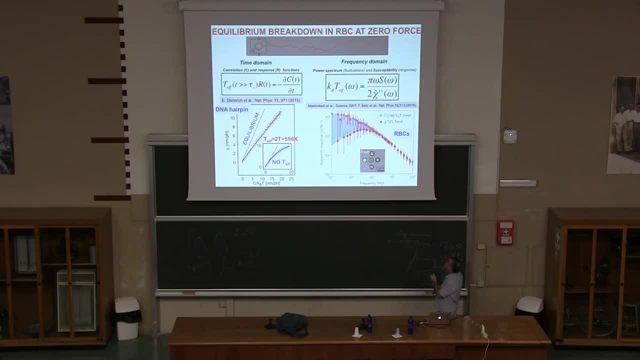 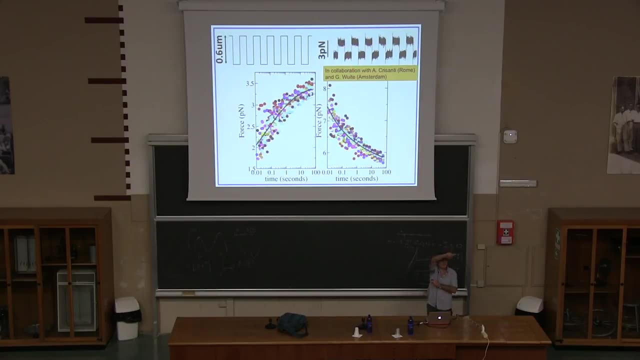 I am doing the experiments now at every force in a very wide range of conditions, and we want to measure, not in frequency space, but it is basically the same. now we are doing the experiments. this is a collaboration with Andrea Bisanti, which is somewhere there, and Heijswoude in Amsterdam. 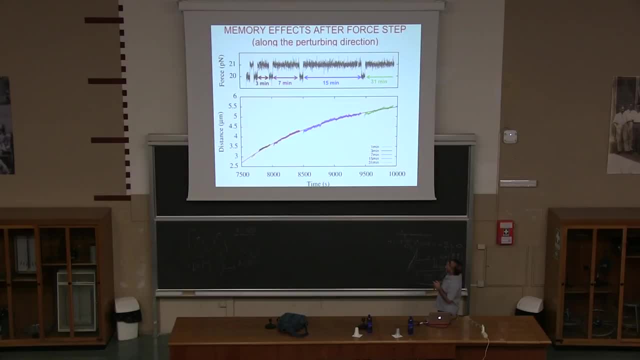 we are trying to apply our theory in this, and you can also do experiments on memory effects. I won't show you much about this, but this has to be properly designed, because we cannot quench temperature. we can just change the force, and then this adds some sort of problems. 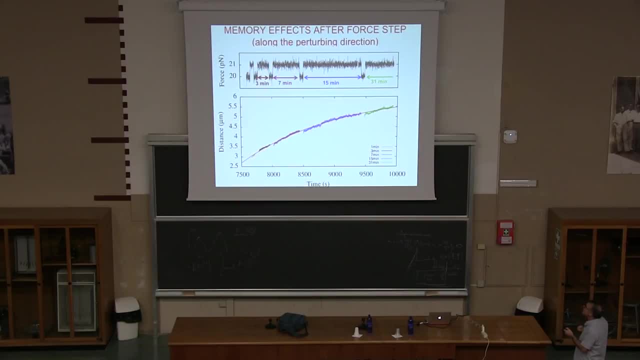 but there are strong memory effects, so you do jumps in force from 20 piconewtons to 21 and then you measure the response in different times. you can superimpose them in a single curve. it remembers how much you deform previously. these are the conclusions. 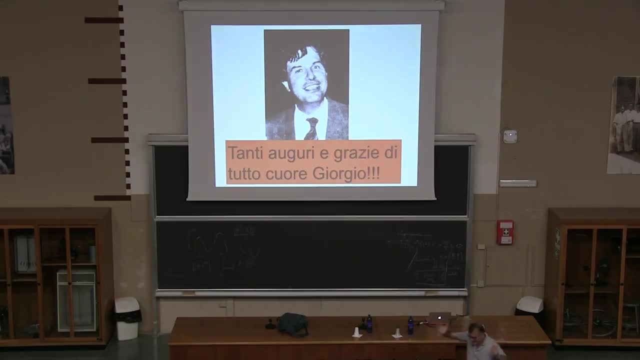 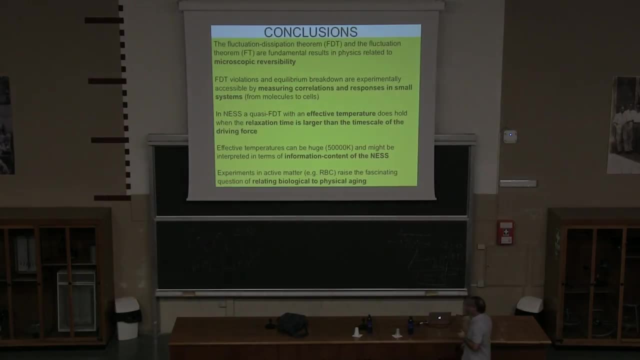 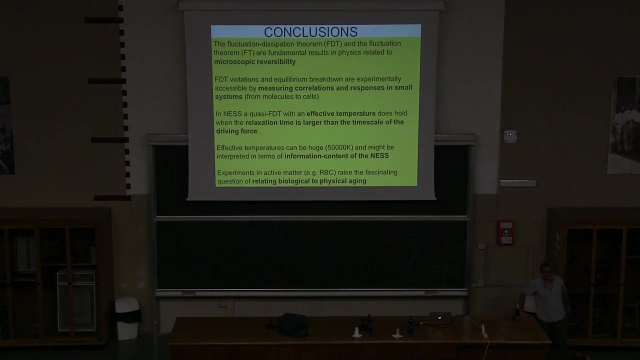 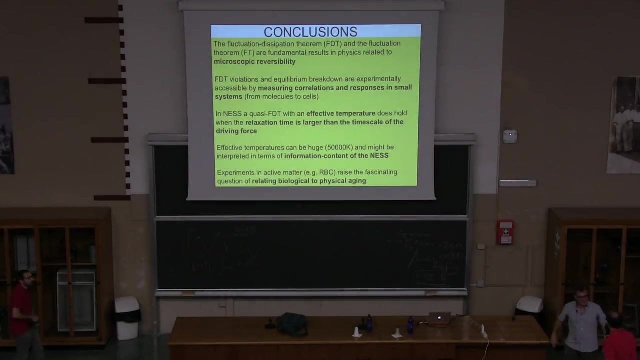 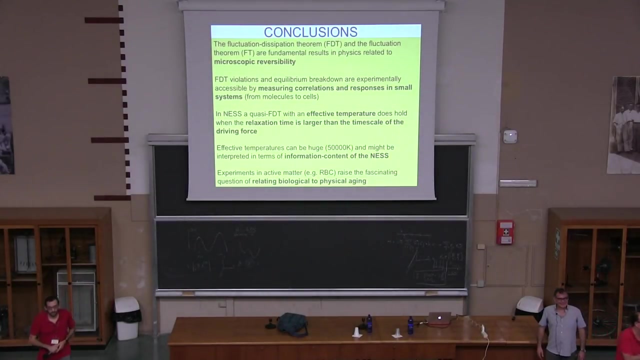 but of course this talk was in memory and dedication. sorry, sorry, dedication to John everybody. thank you vào Healthcare. thank you very much for your interesting talk. we have time for a couple of questions. sorry, Giorgio. no, because most memories I remember, not because you are not there. 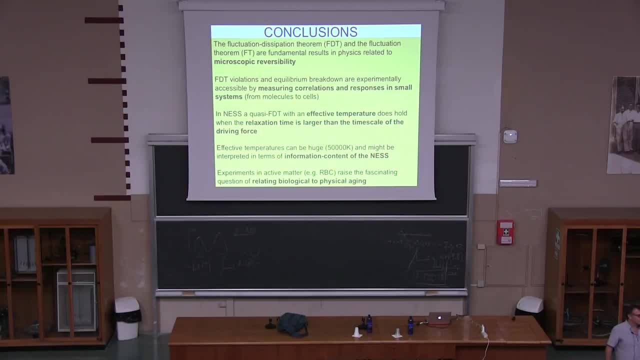 could you, were you able to correlate the age of the? so can you somehow control the age of the red blood cell and see if there is a correlation with the, with the fluctuation dissipation parameter, etc. so is that? yeah, that's a good question, it's. 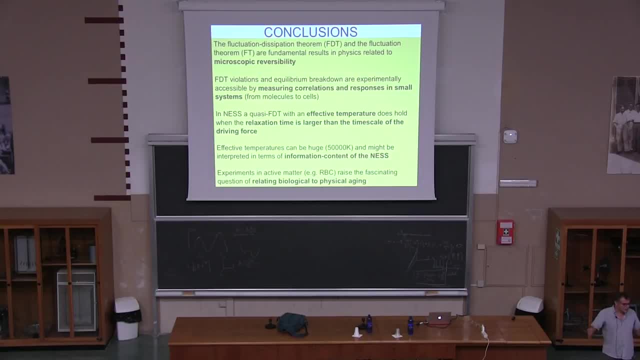 very. that would be very nice because you could prepare your sample at different ages, right. but the problem is that when you take a sample of blood, this is very difficult to you take blood because they those are from healthy donors, so this blood is real blood. so they come at different stages. they have been 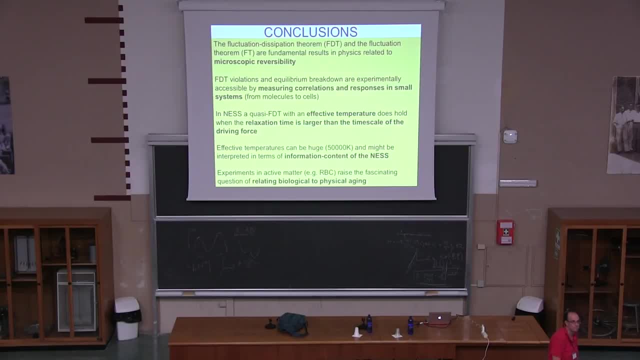 producing the splint bone marrow at different ages. you cannot, it's very difficult to separate this age and there are ways, but it's not trivial and and it's hard to see that. what you could do anyway, you could take a population which is more aged than other one and start to crop it and see whether there is a 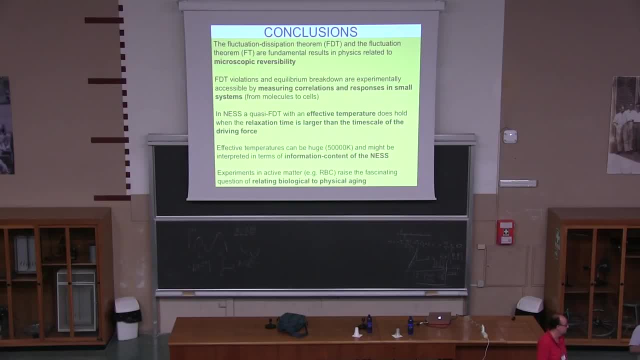 change. so even if you cannot separate by ages, you could still see if there is a, let's say, an age, intrinsic age in a population. okay, so you mentioned very fast that in some of the equivalents between constant force and and constant length. so is it established or is which? 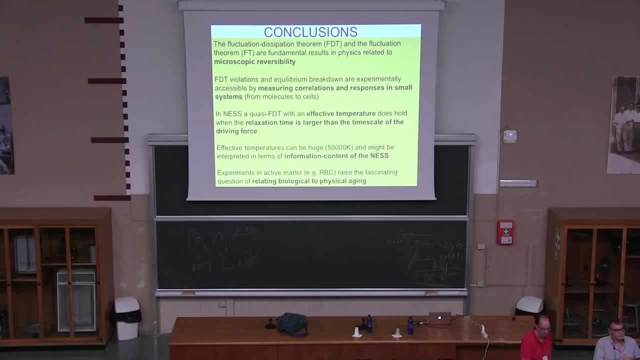 is the origin, or so, so is it the finiteness of the system that induces this. so it's known that masthew means كن segunda قطع, تمنślę. force, let's say, and constant extension are not the same. 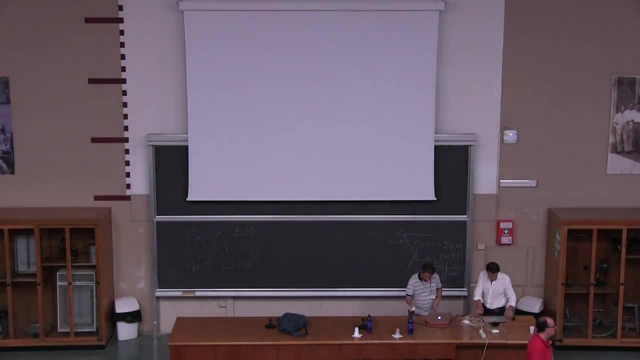 And in magnetic systems it's the same. Constant magnetic field and constant magnetization is not the same. What I said is that at the experimental level I can do in my case, whether in the magnetic case or in the electric case, it's extremely difficult. So in my case, of course, I see. 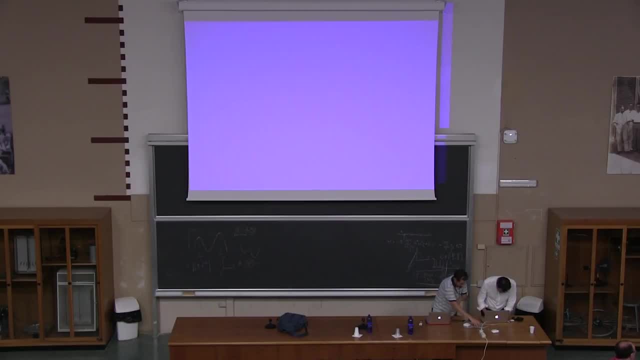 strong differences. However, if these relations, fluctuation, dissipation zone- are generic and hold whenever you have an unequilibrium system, it should not depend specifically on which parameter you really control and which one you don't control, So which one is fluctuating or which one it is not, which means which ensemble you are. 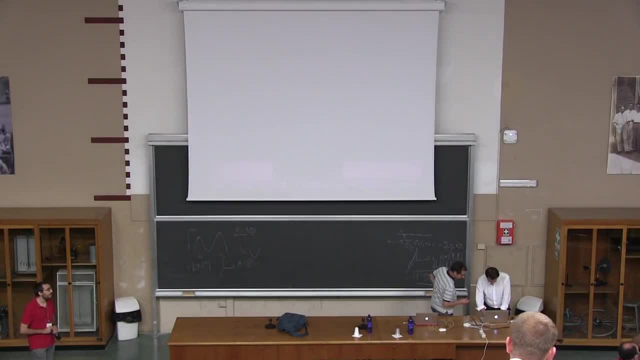 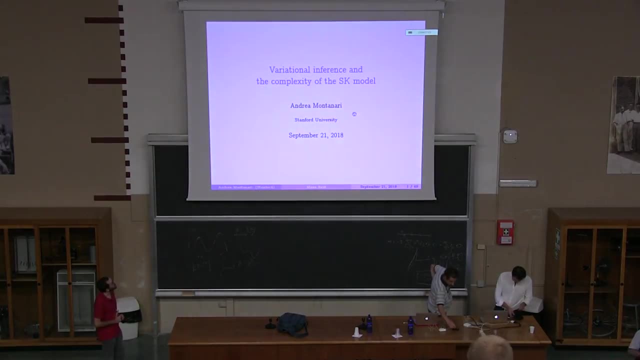 At the end of the day, it's the same. Although the specific mathematical form of the fluctuation dissipation theorem, or the form of the entropy production, or whatever it is, it depends on the ensemble, And that's what we have seen, that all ensembles. 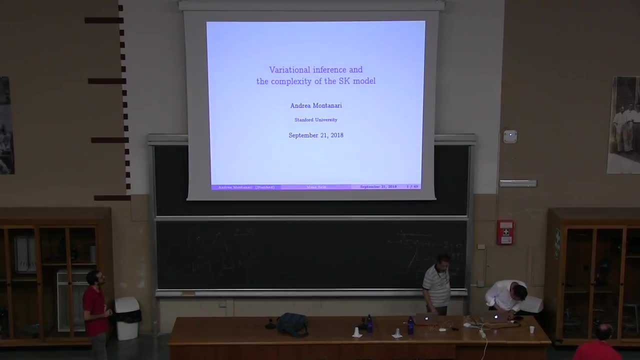 are equivalent in the sense that the relations hold, but they give you different results, of course. Okay, let's thank Félix again for this third talk.